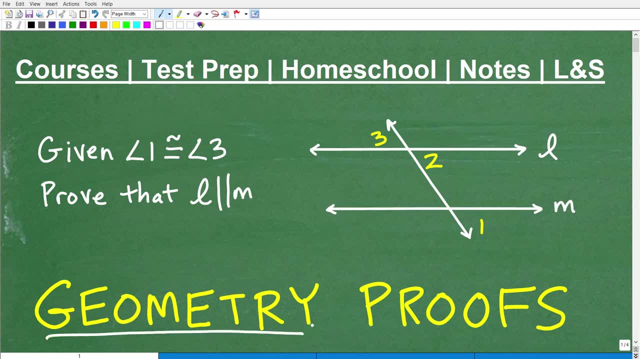 Okay, let's talk about geometry proofs, And these are problems that you typically start to encounter at the high school level. So, if you're taking high school geometry and your teacher is giving you problems, let's say something like: prove this or prove that. Matter of fact, let's go ahead and take a look at this example. This will kind of, you know, clarify what I'm talking about. So, given that angle one is congruent to angle three- and I'm talking about what's going on in this figure right here- we want to prove that. 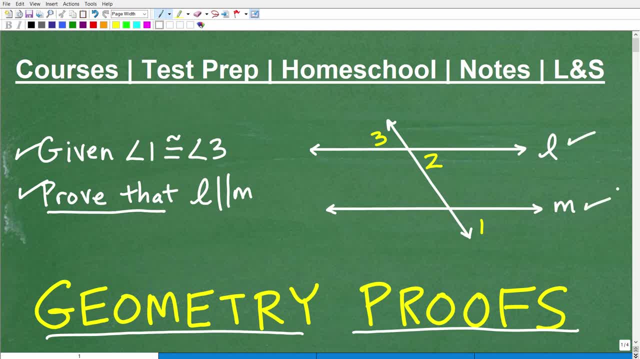 We want to prove that line L is parallel to line M. Now, these two lines appear to be parallel, but we can't write this down and be like: well, line L looks to be parallel to line M, therefore L and M are parallel. Well, of course, we're going to need an actual, concrete justification, some proof, And this is no different than you know how, like a lawyer or an attorney you know is talking in court, right, They're trying to convince. 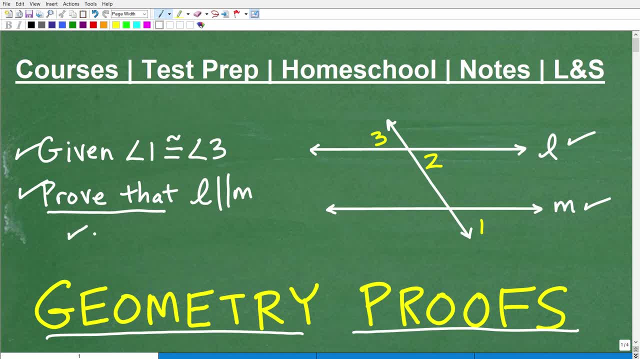 a jury of something They're saying. you know this, then this, then therefore it must be this: you know, believe in what I'm telling you, because here is the proof right To you. know, say that my client is innocent or guilty, whatever the case might be. Oh, of course you know, if your attorney is trying to say that you're guilty, you got problems. But anyways, hopefully you'll understand the idea that a proof is proving something. Okay, so you need to kind of put that kind of thinking cap on that. All right, how do I justify something? Well, in 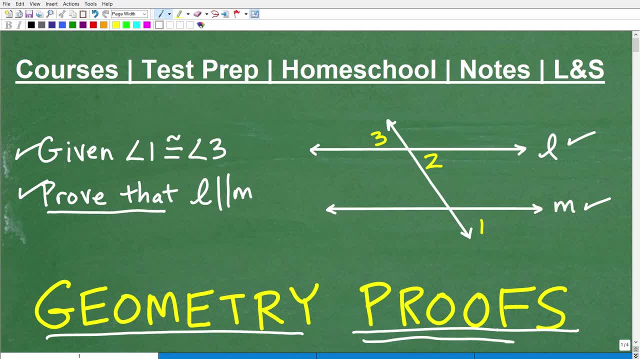 mathematics, you have to follow very specific rules, And the rules, or the kind of the structure we're going to be using at the high school level, in terms of high school level geometry proofs is something called deductive logic. Okay, so I'm going to be kind of going over what are very common type of proofs that high school students face when they take geometry. Now I will say this: most students hate doing these type of problems, But just remember that there's not one way to prove something. Okay, you could do a nice. 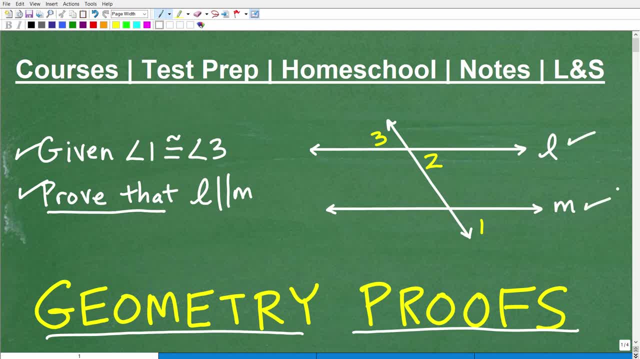 We want to prove that line L is parallel to line M. Now, these two lines appear to be parallel, but we can't write this down and be like: well, line L looks to be parallel to line M, therefore L and M are parallel. Well, of course, we're going to need an actual, concrete justification, some proof, And this is no different than you know how, like a lawyer or an attorney you know is talking in court, right, They're trying to convince. 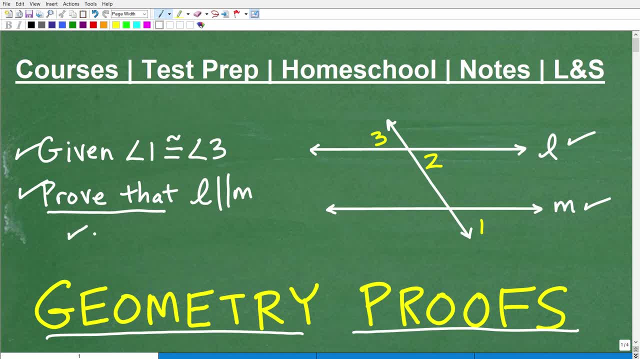 a jury of something They're saying. you know this, then this, then therefore it must be this: you know, believe in what I'm telling you, because here is the proof right To you. know, say that my client is innocent or guilty, whatever the case might be. Oh, of course you know, if your attorney is trying to say that you're guilty, you got problems. But anyways, hopefully you'll understand the idea that a proof is proving something. Okay, so you need to kind of put that kind of thinking cap on that. All right, how do I justify something? Well, in 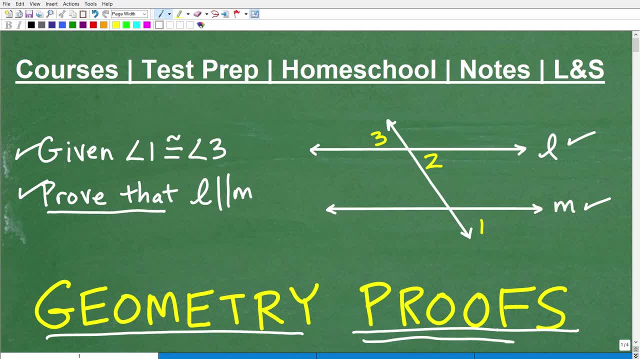 mathematics, you have to follow very specific rules, And the rules, or the kind of the structure we're going to be using at the high school level, in terms of high school level geometry proofs is something called deductive logic. Okay, so I'm going to be kind of going over what are very common type of proofs that high school students face when they take geometry. Now I will say this: most students hate doing these type of problems, But just remember that there's not one way to prove something. Okay, you could do a nice. 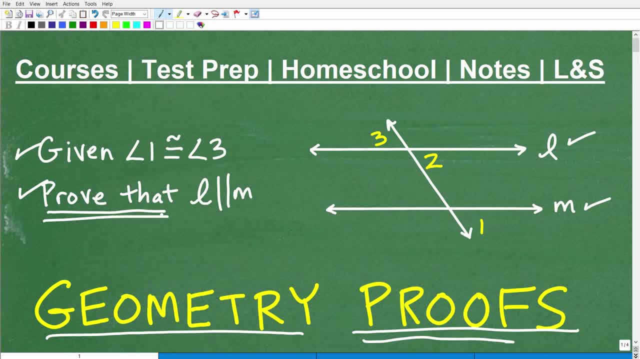 proof. It might be different than what your teacher would do, but it could still be technically correct. But you do have to follow very specific rules, And that's what this video is going to be about. But I will say one thing to this concept of proving things is the essence of mathematics. My degree is in theoretical mathematics And at the university level most of the problems that I did- well, a huge majority of them- would be things that had to deal with proving stuff prove this show that. So this is truly kind of the essence of 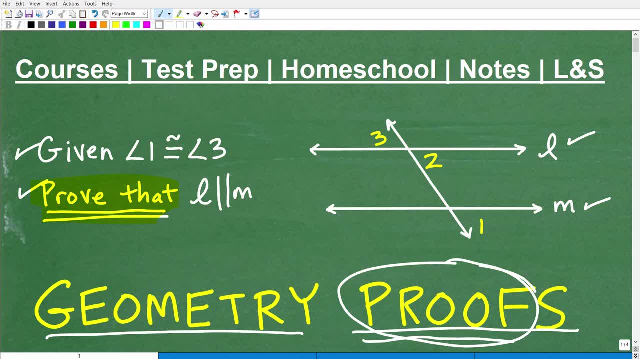 essence of mathematics, if you're just curious about that. but we're going to get to all this in just one second matter of fact. if you think you can actually construct a proof for this, that would be super impressive. without seeing what i'm doing, i'll talk about all the details here in a 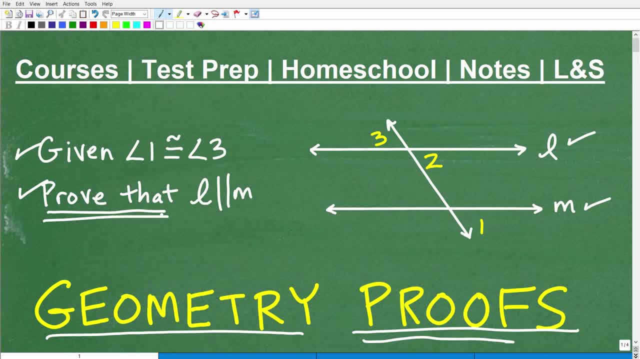 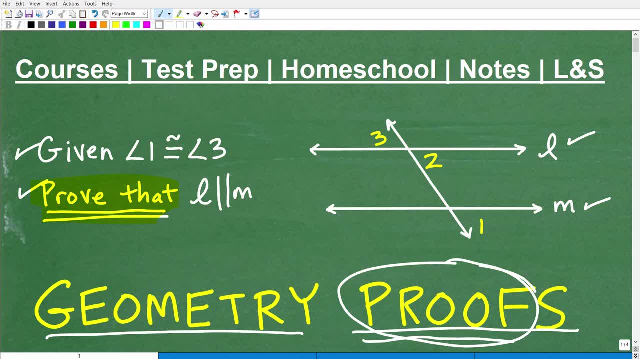 essence of mathematics, if you're just curious about that. but we're going to get to all this in just one second matter of fact. if you think you can actually construct a proof for this, that would be super impressive. without seeing what i'm doing, i'll talk about all the details here in a 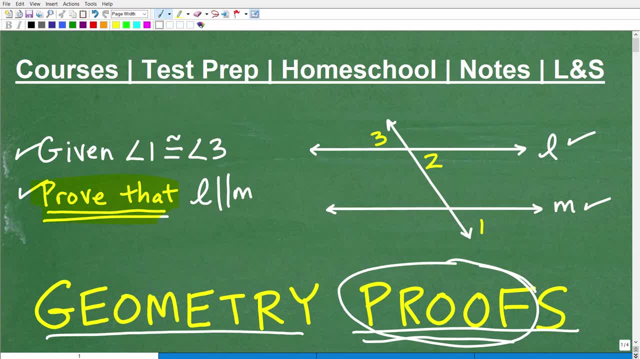 second, but first let me quickly introduce myself. my name is john. i'm the founder of tc math academy. i'm also a middle and high school math teacher. i've been teaching math for decades and i'm telling you right now: if you're struggling in mathematics, please don't give up. there is hope, what you need. 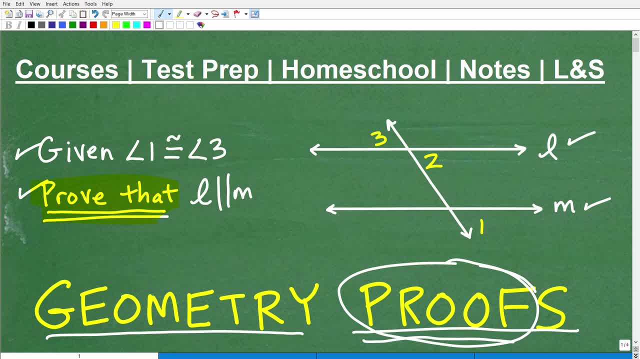 is great math instruction: clear, understandable, comprehensive. so if you're at the middle school, high school or even college level, check out my math help program. you can find it a link. you can find it by following the link in the description. if you are watching this video, i assume you are. 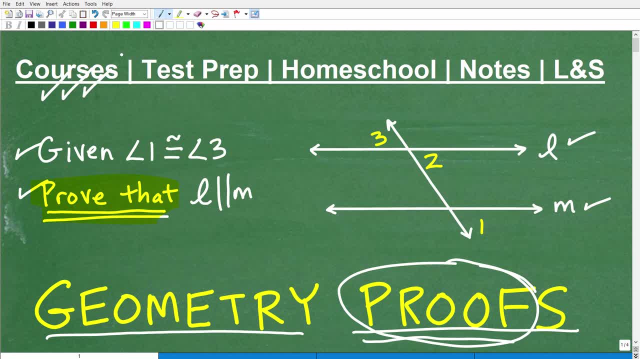 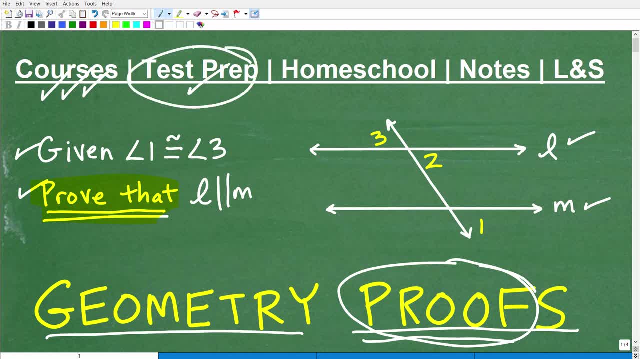 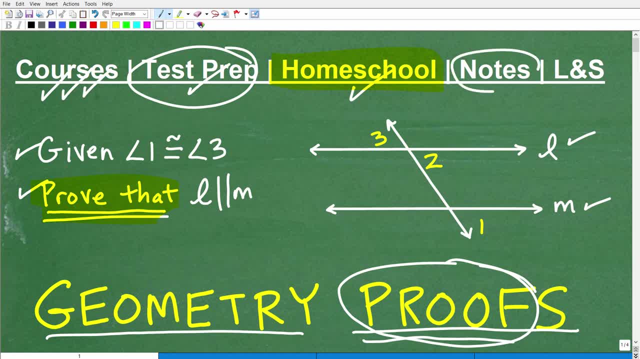 programs for middle and high school level mathematics. if you need a pair of math notes, i'm going to leave links to my math notes in the description of this video, but hopefully you have your own great notes. okay, this is one of the keys to be successful in mathematics, and if this video 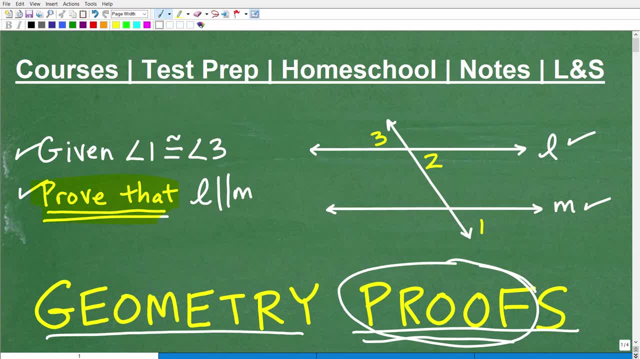 second, but first let me quickly introduce myself. my name is john. i'm the founder of tc math academy. i'm also a middle and high school math teacher. i've been teaching math for decades and i'm telling you right now: if you're struggling in mathematics, please don't give up. there is hope, what you need. 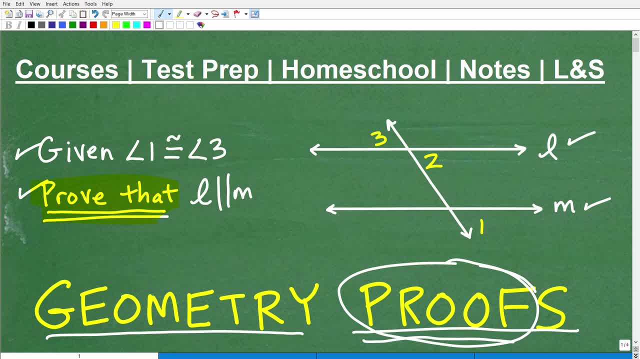 is great math instruction: clear, understandable, comprehensive. so if you're at the middle school, high school or even college level, check out my math help program. you can find it a link. you can find it by following the link in the description. if you are watching this video, i assume you are. 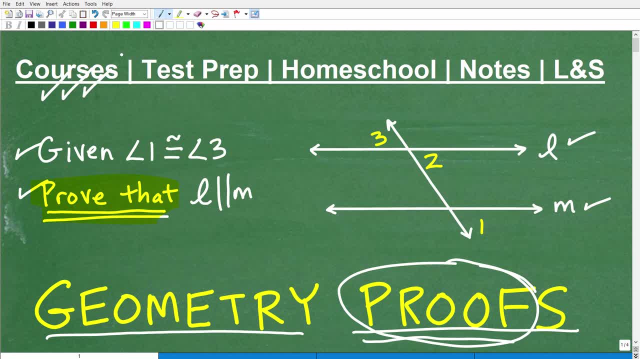 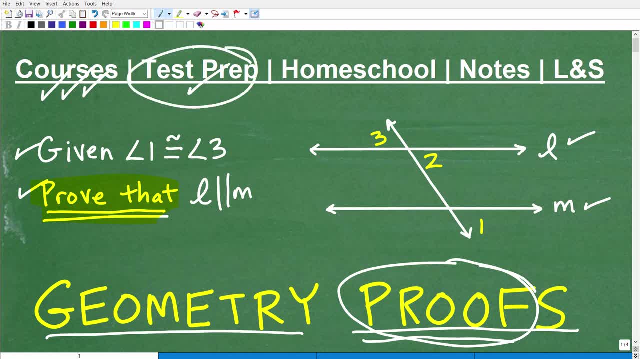 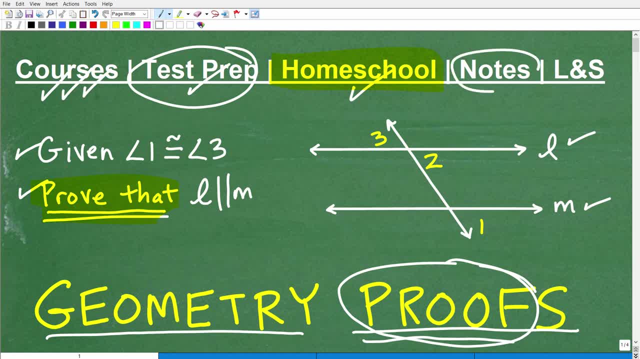 programs for middle and high school level mathematics. if you need a pair of math notes, i'm going to leave links to my math notes in the description of this video, but hopefully you have your own great notes. okay, this is one of the keys to be successful in mathematics, and if this video 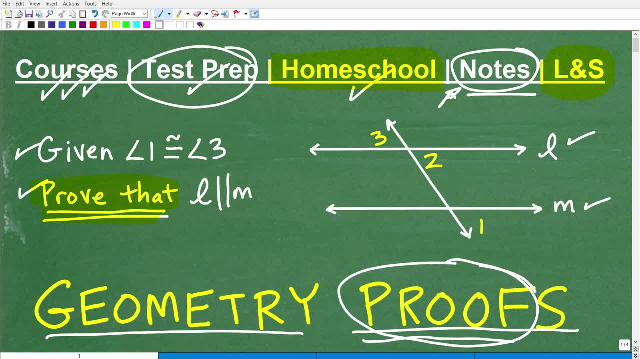 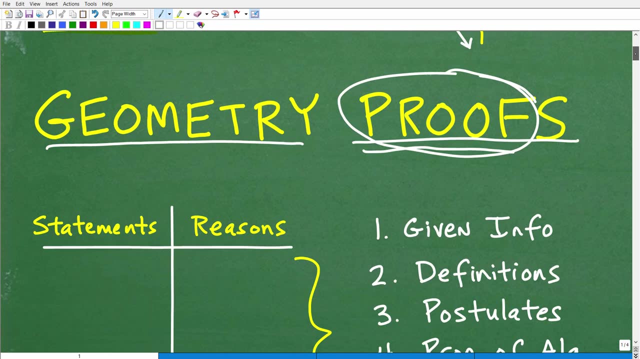 helps you out. don't forget to like and subscribe. okay, so proves big topic. and for most students- students, uh, you know, taking high school level geometry- they don't like doing these type of problems. so if you're like, yeah, that's me. well, you know, that's what this video was designed to help. 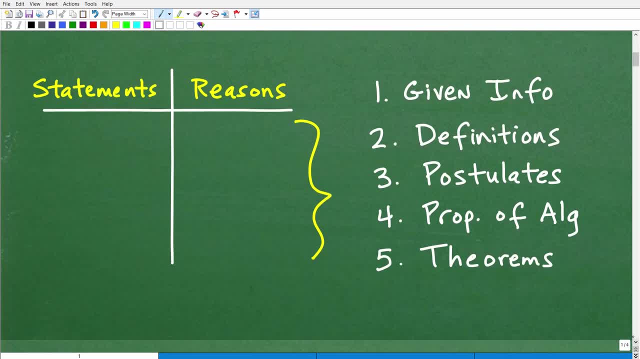 uh, those of you out there are struggling with proofs, but let's take a look at what a proof kind of is going to look like. so what we're going to be doing here is what we call a two column proof. it's the most typical type of format for this level of 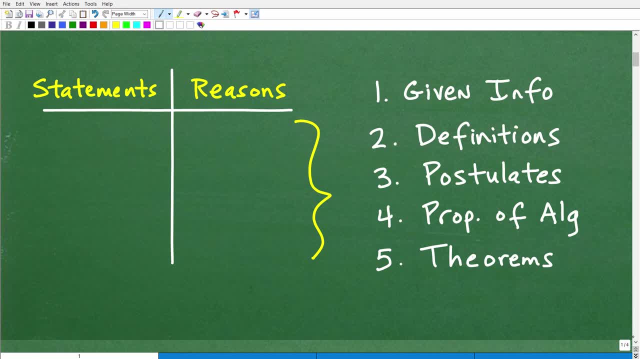 mathematics for what you're going to be dealing with. again, this is, generally speaking, most you have out there taking high school geometry. it's kind of where this video is targeted at, but maybe some of you need to just review uh geometry in general. okay, so a two column proof is uh basically looks. 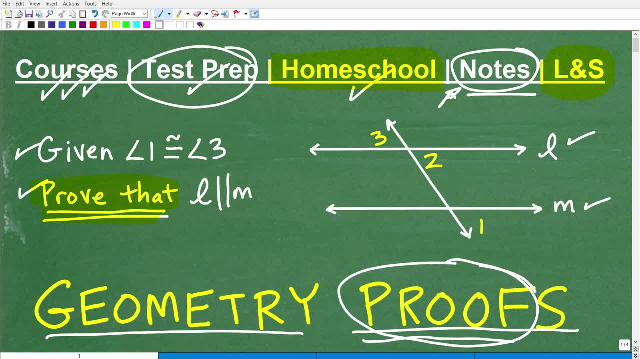 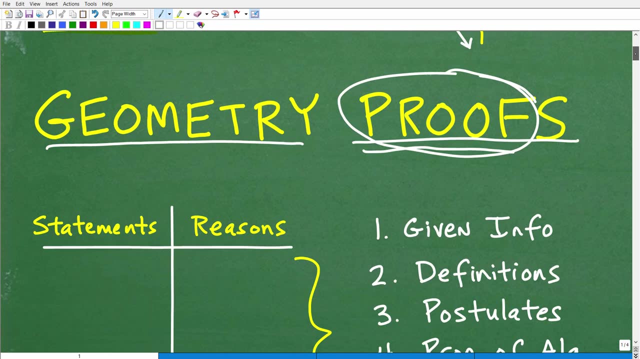 helps you out. don't forget to like and subscribe. okay, so proves big topic. and for most students- students, uh, you know, taking high school level geometry- they don't like doing these type of problems. so if you're like, yeah, that's me. well, you know, that's what this video was designed to help. 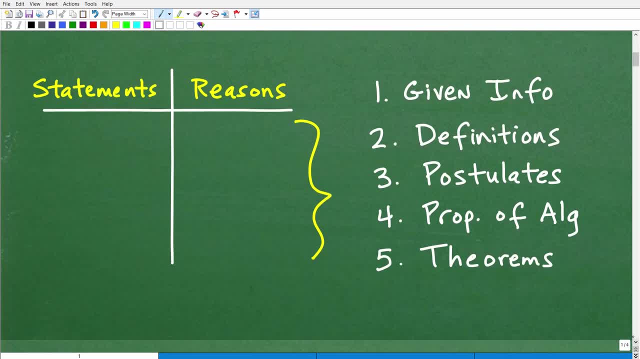 uh, those of you out there are struggling with proofs, but let's take a look at what a proof kind of is going to look like. so what we're going to be doing here is what we call a two column proof. it's the most typical type of format for this level of 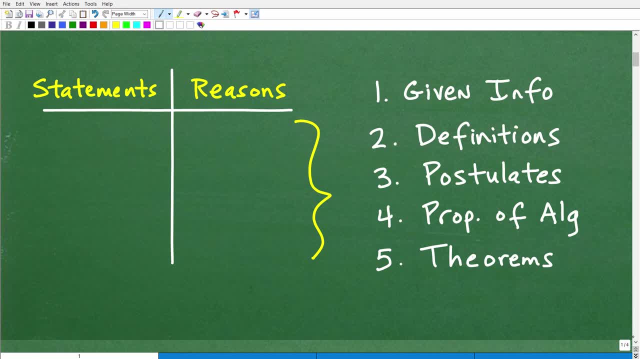 mathematics for what you're going to be dealing with. again, this is, generally speaking, most you have out there taking high school geometry. it's kind of where this video is targeted at, but maybe some of you need to just review uh geometry in general. okay, so a two column proof is uh basically looks. 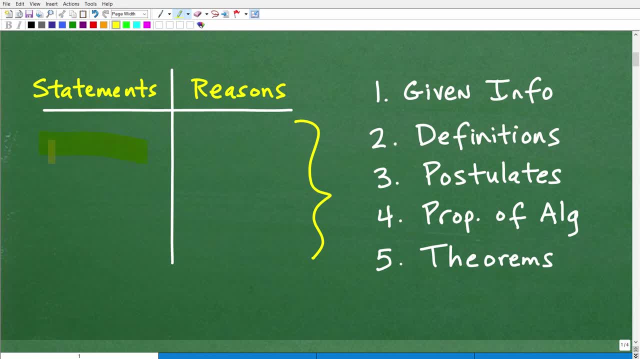 like this: okay, there's two columns here. you're going to make a statement, you're going to say something, then you're going to back that statement up. you're going to give a reason why you're saying that or justify that. so you're going to make a statement and you're going to give a reason then. 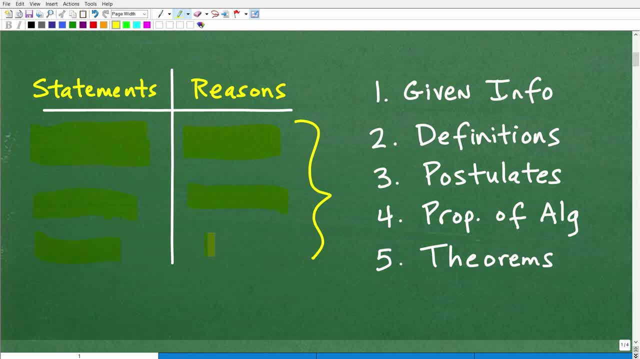 you're going to make another statement and then you're going to give another reason, but the statements have a certain flow. okay, what you're trying to do is go and argue. okay, you're trying to prove your final point. okay, so you're trying to prove something, and it's no different than saying: 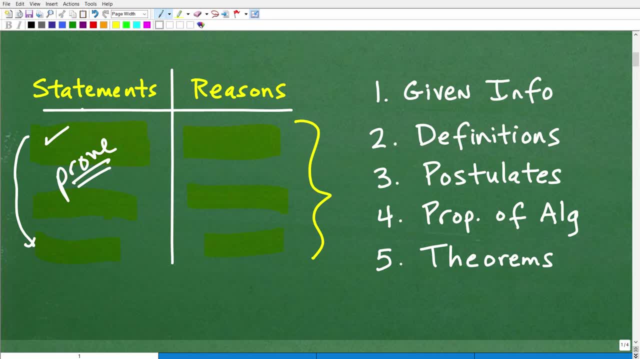 you know, to your best friend: hey, uh, uh. you know you're trying to, let's say, convince them of something and you're debating or arguing about something. you say: well, don't you agree that this happened? they'll say: oh yeah, okay, yeah, that happened, all right, boom right. so you say: okay. 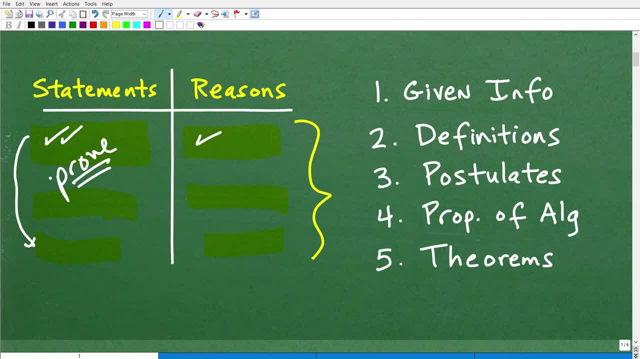 that happened. all right, then you. then you try to walk them to your next point. i'm pretty sure you know um understands what i'm saying. maybe it's your brother or sister or your boyfriend or girlfriend. whatever the case might be, you're like: okay, what about this? now, this happened. 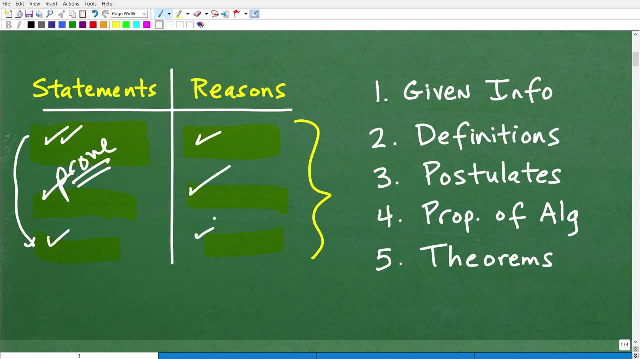 right, okay, yeah, yeah, or that happened too, boom. so you're trying to step by step, logically, you know, get to a certain conclusion. okay, this is the idea in doing a proof, but again with those very specific rules, because, uh, when we're dealing with, uh, geometric proofs, all right, so we're 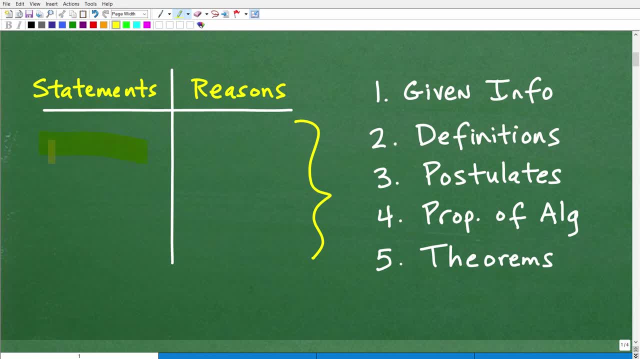 like this: okay, there's two columns here. you're going to make a statement, you're going to say something, then you're going to back that statement up. you're going to give a reason why you're saying that or justify that. so you're going to make a statement and you're going to give a reason then. 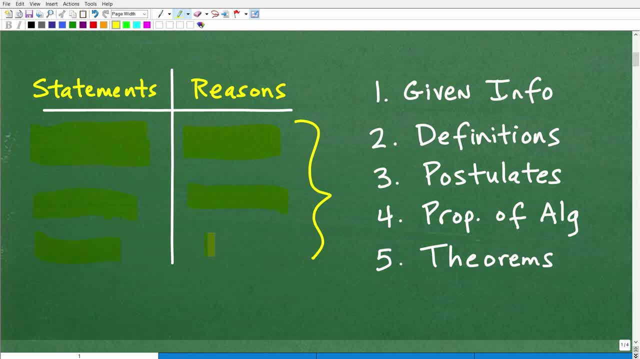 you're going to make another statement and then you're going to give another reason, but the statements have a certain flow. okay, what you're trying to do is go and argue. okay, you're trying to prove your final point. okay, so you're trying to prove something, and it's no different than saying: 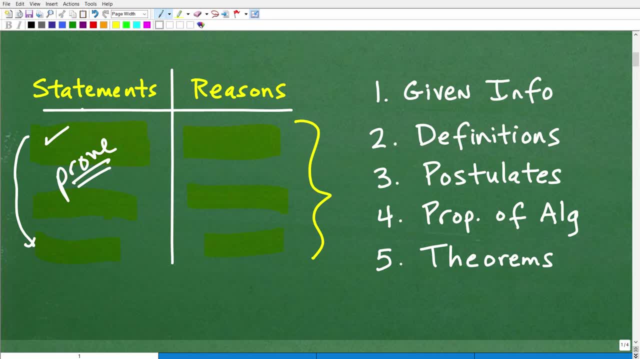 you know, to your best friend: hey, uh, uh. you know you're trying to, let's say, convince them of something and you're debating or arguing about something. you say: well, don't you agree that this happened? they'll say: oh yeah, okay, yeah, that happened, all right, boom right. so you say: okay. 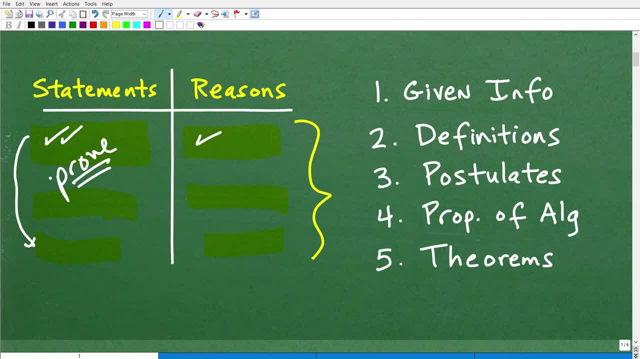 that happened. all right, then you. then you try to walk them to your next point. i'm pretty sure you know um understands what i'm saying. maybe it's your brother or sister or your boyfriend or girlfriend. whatever the case might be, you're like: okay, what about this? now, this happened. 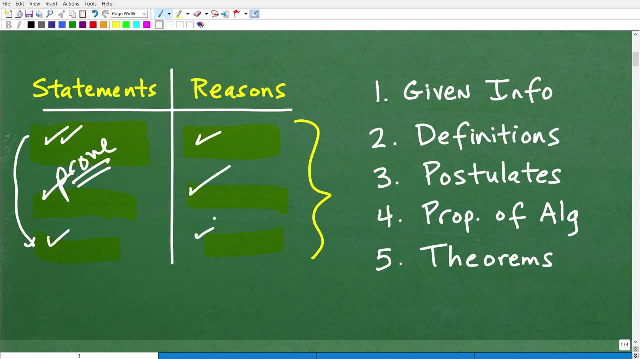 right, okay, yeah, yeah, or that happened too, boom. so you're trying to step by step, logically, you know, get to a certain conclusion. okay, this is the idea in doing a proof, but again with those very specific rules, because, uh, when we're dealing with, uh, geometric proofs, all right, so we're 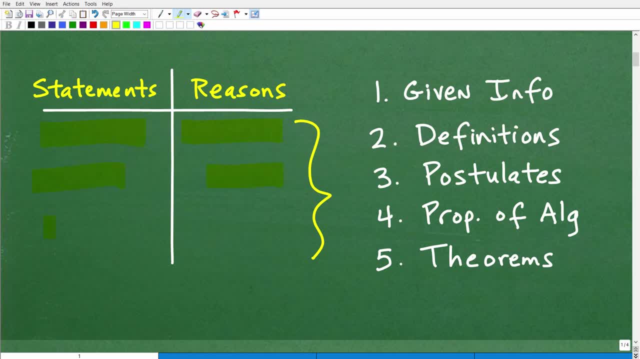 going to give a statement, and then we're going to give a reason and we're going to going to continue to make as many statements and back this up with, uh, with as many reasons, until we reach our final conclusion, until we have proved what we want to prove. now, here's the thing you 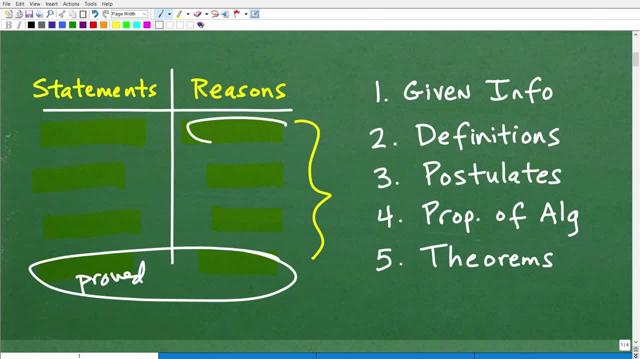 can see, i have some stuff going on over here. the reasons you can list here is the main kind of point. well, one of the main points of this video, the reasons that you can give aren't opinions. you're not going to say uh, uh, don't you think that you know these two angles are uh equal, because they look to be equal. 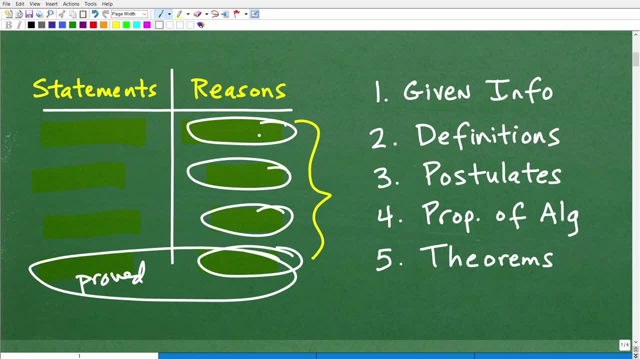 you know, because you know, i measure them on my paper and they look and they are equal. no, you can't give a reason like that. the only reasons you can give- okay in a geometric proof- and this is kind of classic geometry- is the following: one is given information. okay, now what am i talking? 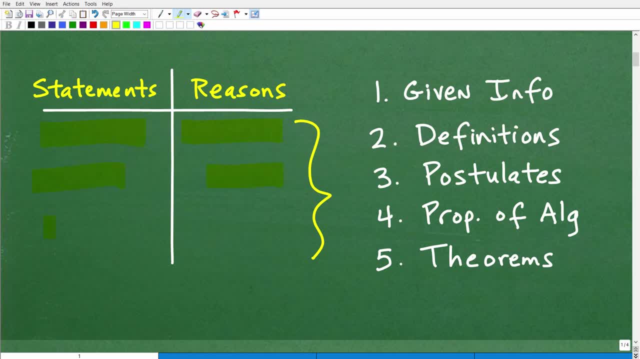 going to give a statement, and then we're going to give a reason and we're going to going to continue to make as many statements and back this up with, uh, with as many reasons, until we reach our final conclusion, until we have proved what we want to prove. now, here's the thing you 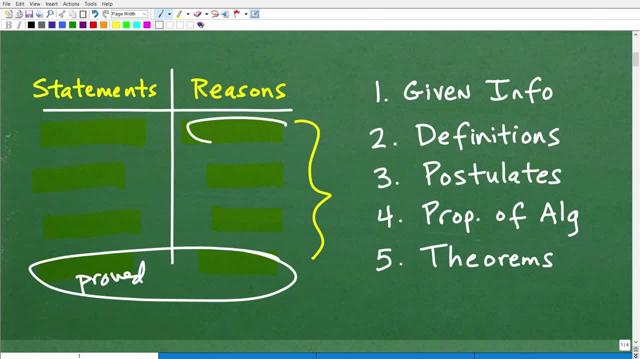 can see, i have some stuff going on over here. the reasons you can list here is the main kind of point. well, one of the main points of this video, the reasons that you can give aren't opinions. you're not going to say uh, uh, don't you think that you know these two angles are uh equal, because they look to be equal. 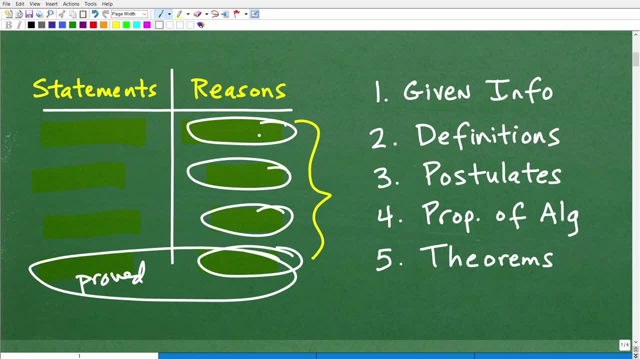 you know, because you know, i measure them on my paper and they look and they are equal. no, you can't give a reason like that. the only reasons you can give- okay in a geometric proof- and this is kind of classic geometry- is the following: one is given information. okay, now what am i talking? 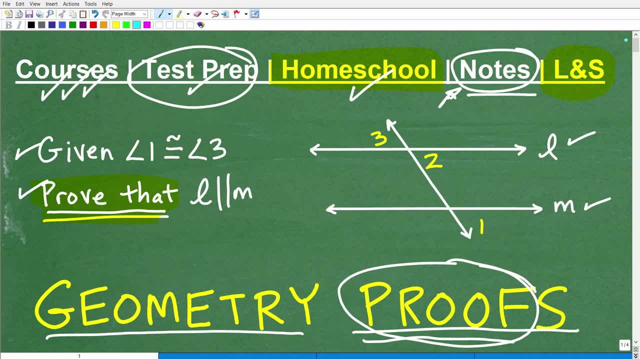 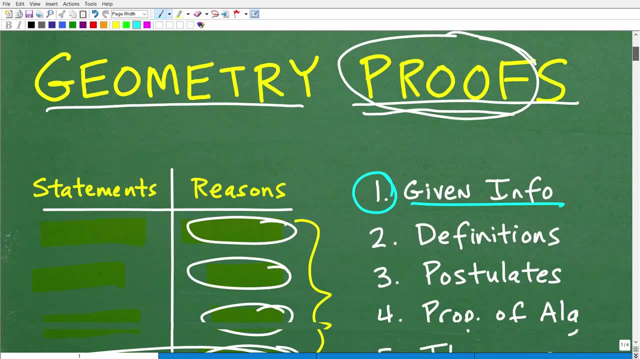 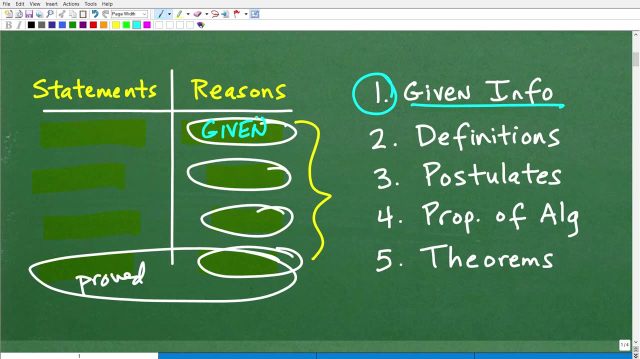 about given information. well, let's go back up here. in this proof i told you, given that angle one is congruent to angle three. i gave you that information so you can justify that. and, given information, your first statement is typically almost always going to be: you're going to kind. 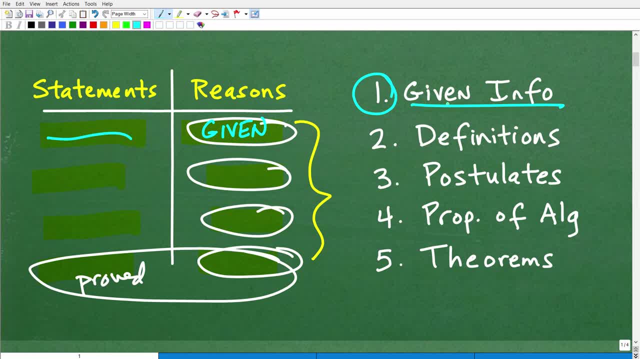 of repeat that given information. okay, so that's one thing you can. you can, uh, give, but oftentimes you can use this given information, you know, in other um statements throughout the proof, if you need to. so that's one allowable justification for a statement okay, or a reason you can back it up. the second thing is definitions: okay, so definition so. 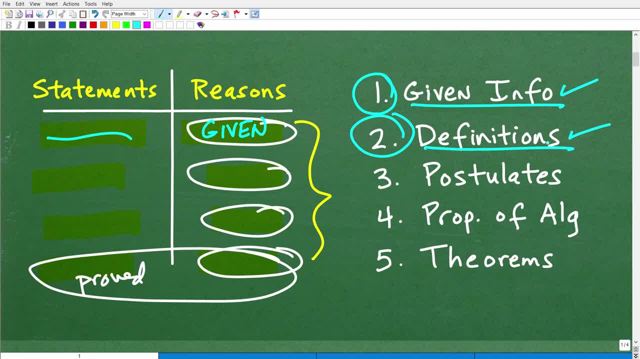 like a triangle, has a specific definition of what it is right, a circle or parallel lines. okay these, they have very specific mathematical definitions and this is where your notes come in big time, if you're not taking like notes in any math course, but especially in geometry, because you're going to be learning a ton of theorems, properties, 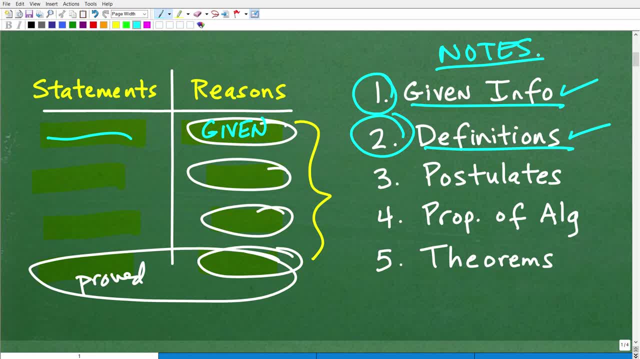 postulates, axioms, corollaries, there's even these things called lemmas. There are a ton and ton and ton. I mean like it can just add up hundreds and hundreds and hundreds of these little definitions, postulates. You need to be highly organized and be able to call upon. 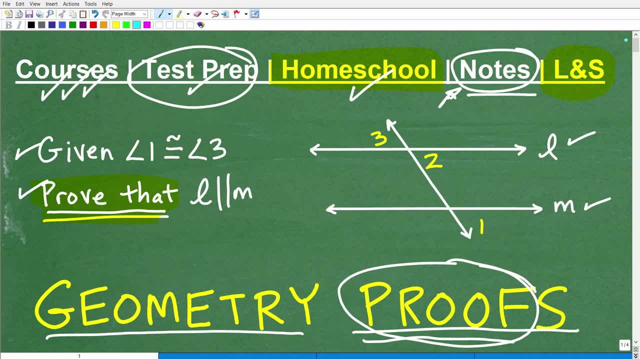 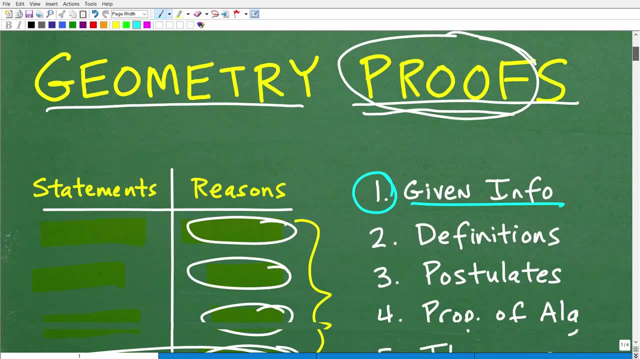 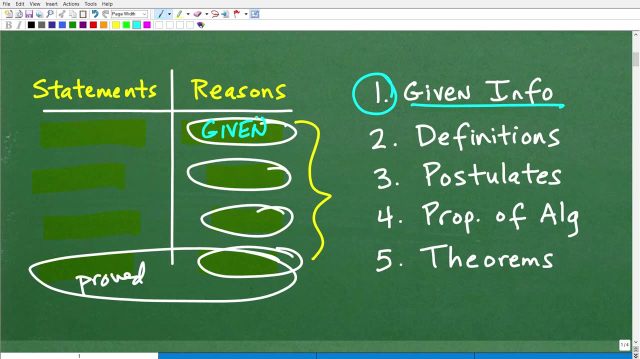 about given information. well, let's go back up here. in this proof i told you, given that angle one is congruent to angle three. i gave you that information so you can justify that. and, given information, your first statement is typically almost always going to be: you're going to kind. 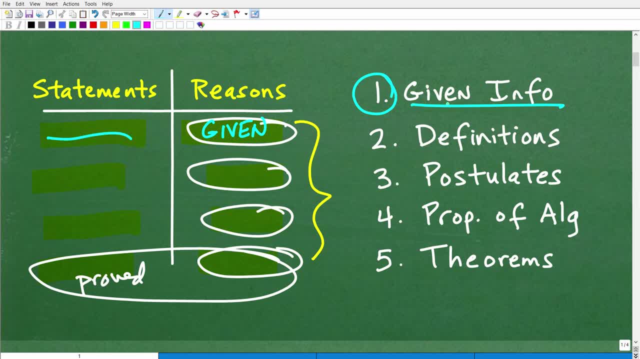 of repeat that given information. okay, so that's one thing you can. you can, uh, give, but oftentimes you can use this given information, you know, in other um statements throughout the proof, if you need to. so that's one allowable justification for a statement, okay, or a reason, uh, you can back it up. the second thing is definitions. okay, so definition so. 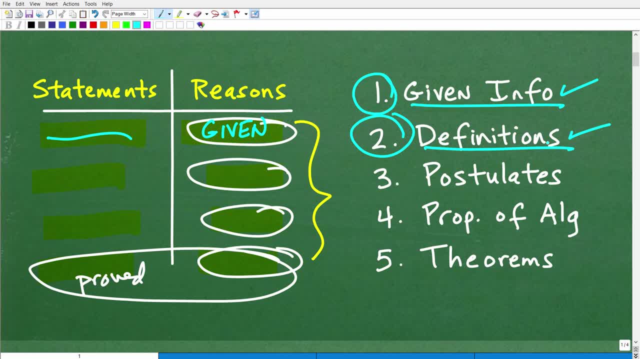 like a triangle, has a specific definition of what it is right, a circle or parallel lines. okay these, they have very specific mathematical definitions and this is where your notes come in big time, if you're not taking like notes in any math course, but especially in geometry, because you're going to be learning a ton of theorems, properties, 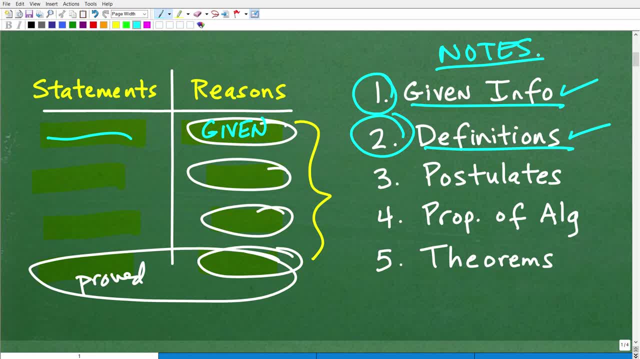 postulates, axioms, corollaries, there's even these things called lemmas. There are a ton and ton and ton. I mean like it can just add up hundreds and hundreds and hundreds of these little definitions, postulates. You need to be highly organized and be able to call upon. 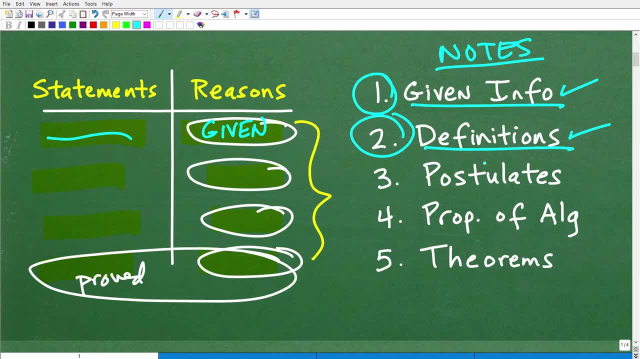 these okay, And this is where I think we're most students struggle with and in terms of geometry course because they're not as good as note takers, as they need to be. You need to have super organized notes Now if you need great geometry notes. 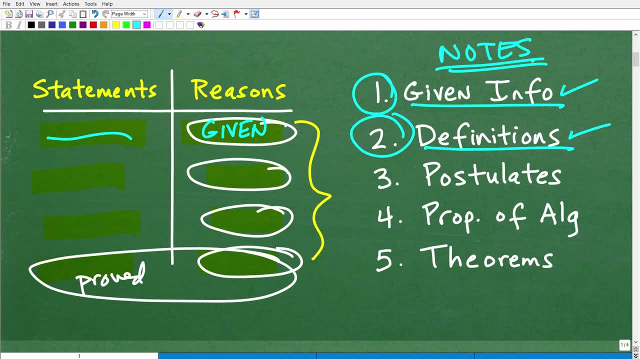 okay, you can check out mine. I'm going to list those in the description of this video. but if you take my geometry course, get access to it. you're going to have access to, like, all my masterwork. okay, that are going to have. 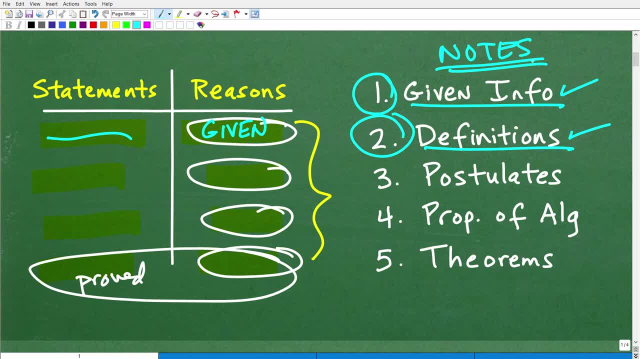 the notes and a ton more, But you need to have access to all the stuff that you've learned up to a particular point in your math course. okay, So that's definitions. Now that goes along with postulates. okay, So a postulate. 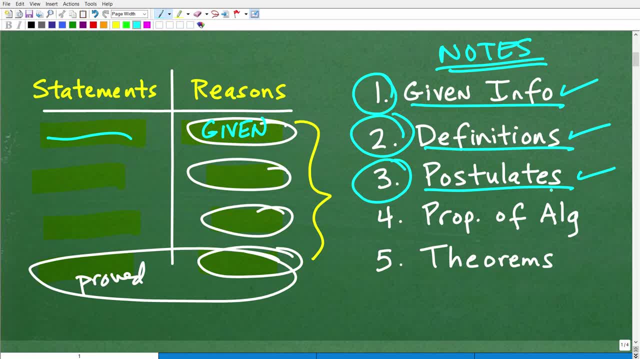 right is different than a theorem, okay. A postulate, basically, is something that we are kind of given. We prove theorems, okay. Postulates are kind of given to us. They're like there's another thing in mathematics called axioms. 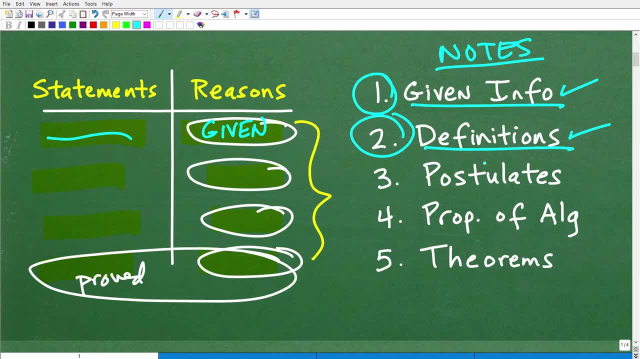 these okay, And this is where I think we're most students struggle with and in terms of geometry course because they're not as good as note-takers- as they need to be. You need to have super organized notes Now if you need great geometry notes. 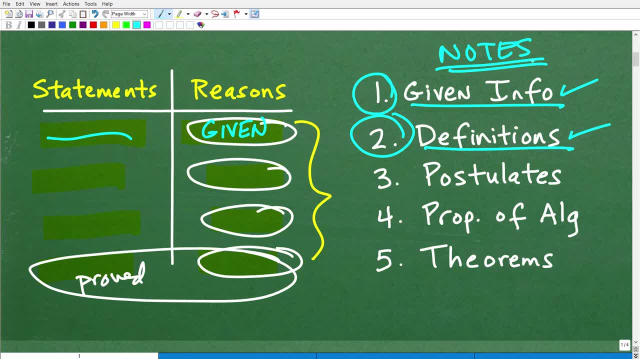 okay, you can check out mine. I'm going to list those in the description of this video. but if you take my geometry course, get access to it. you're going to have access to, like, all my masterwork. okay, that are going to have. 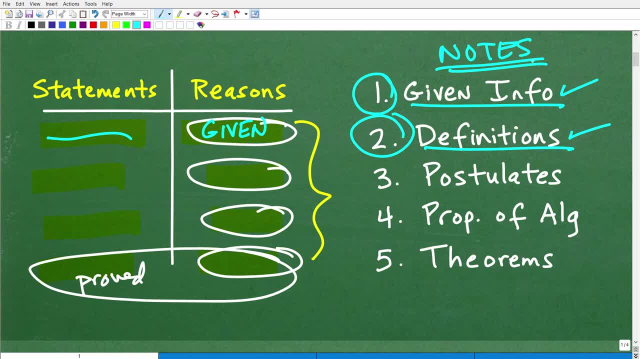 the notes and a ton more, But you need to have access to all the stuff that you've learned up to a particular point in your math course. okay, So that's definitions. Now that goes along with postulates. okay, So a postulate. 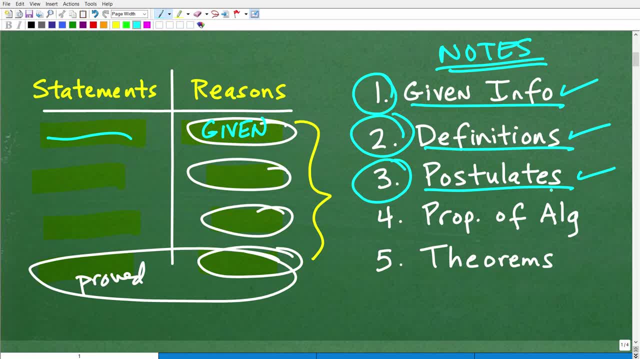 right is different than a theorem, okay. A postulate, basically, is something that we are kind of given. We prove theorems, okay. Postulates are kind of given to us. They're like there's another thing in mathematics called axioms. 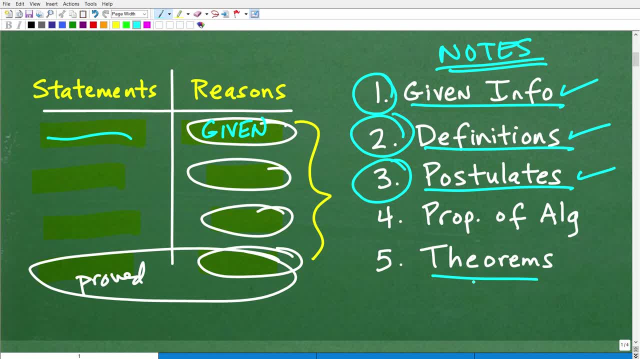 We just assume them to be true, okay, Theorems we actually can prove. Now, just I'm kind of skipping over this here for a second, Just so you can kind of get this idea of theorems. you probably know what this is. 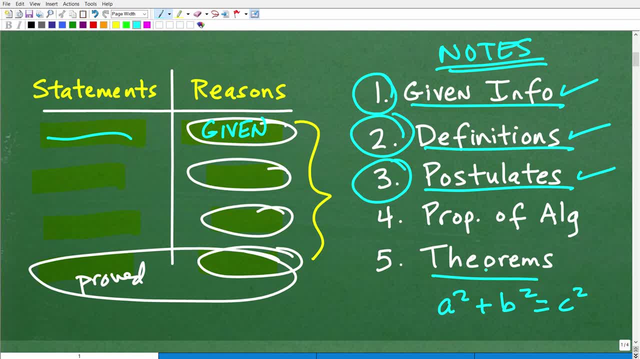 b squared plus b squared is equal to c squared. That's the Pythagorean theorem. okay, That can be proved. We can actually do a nice justification to prove that particular theorem, okay, But a postulate are just: these are things in mathematics that we just kind of 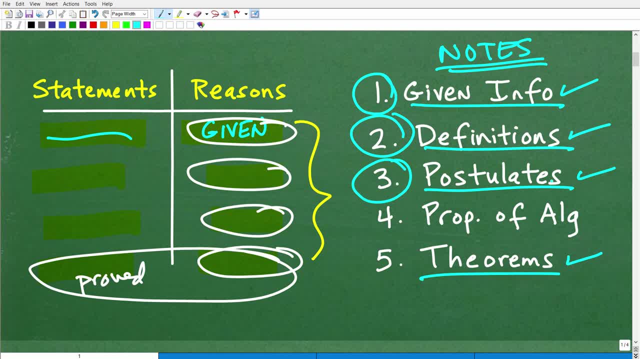 assume to be true, and there's another kind of word that goes for them, like axioms. okay, But postulates are typically- this word is used pretty heavily in geometry- Okay, so let's go on to our next reason here, and that's the properties of algebra and congruence. 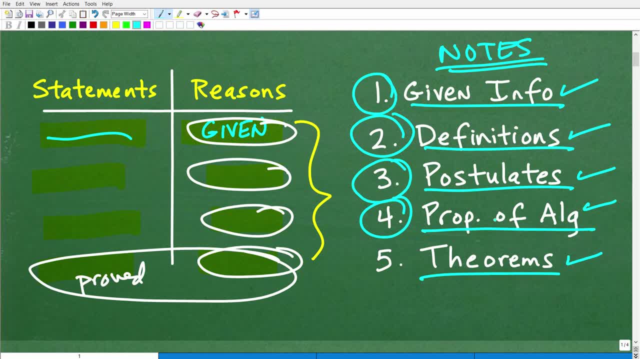 I'm going to show you some examples of what this is, but this is. there's a lot of these as well. okay, There's a ton of these, a lot of these, there's a lot of these. and, of course, there's a ton of theorems which I explained. 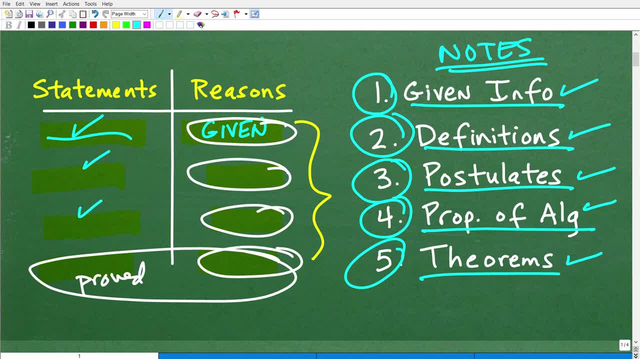 So anytime you give a statement for a proof, the only thing you can say is that: oh, that's given information. this is a definition, this is a postulate. maybe this is a theorem. that's a definition. So you just can't have a. 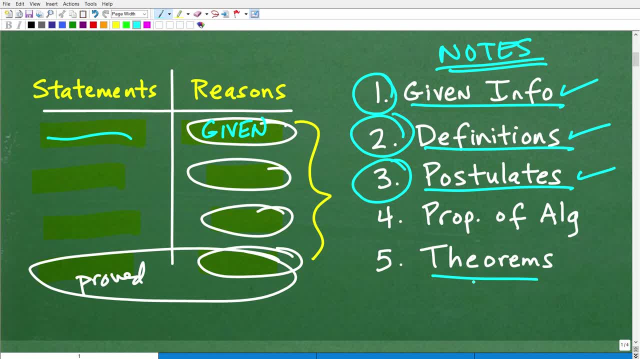 We just assume them to be true, okay, Theorems we actually can prove. Now, just I'm kind of skipping over this here for a second, Just so you can kind of get this idea of theorems. you probably know what this is. 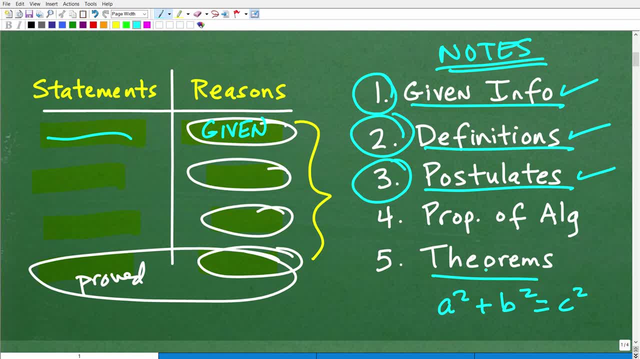 b squared plus b squared is equal to c squared. That's the Pythagorean theorem. okay, That can be proved. We can actually do a nice justification to prove that particular theorem, okay, But a postulate are just: these are things in mathematics that we just kind of 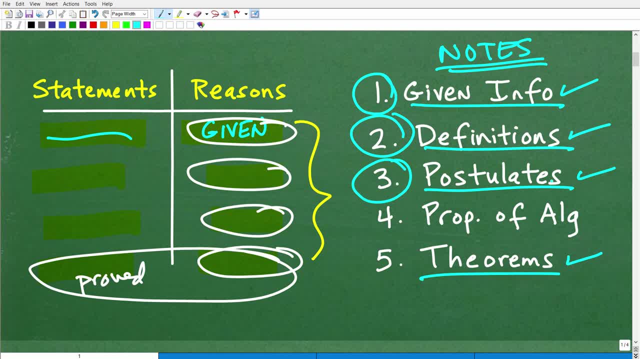 assume to be true, and there's another kind of word that goes for them, like axioms. okay, But postulates are typically- this word is used pretty heavily in geometry- Okay, so let's go on to our next reason here, and that's the properties of algebra and congruence. 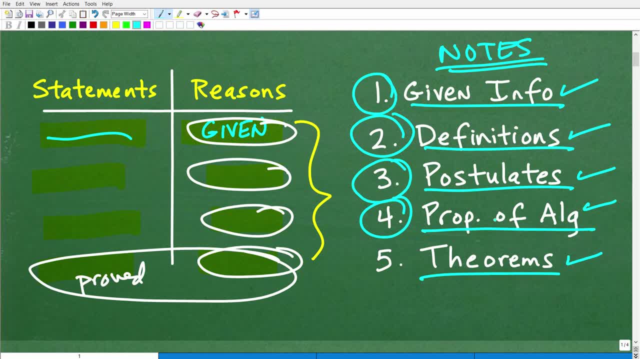 I'm going to show you some examples of what this is, but this is. there's a lot of these as well. okay, There's a ton of these, a lot of these, there's a lot of these. and, of course, there's a ton of theorems which I explained. 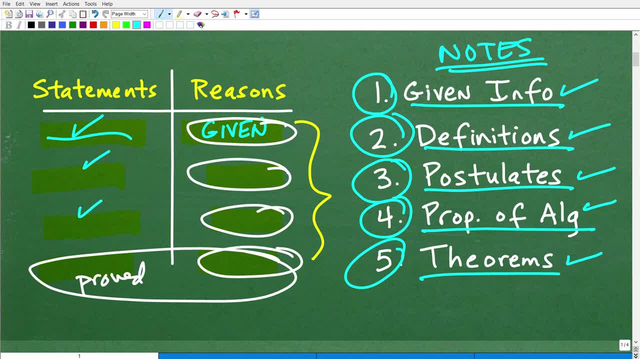 So anytime you give a statement for a proof, the only thing you can say is that: oh, that's given information. this is a definition, this is a postulate. maybe this is a theorem. that's a definition. So you just can't have a. 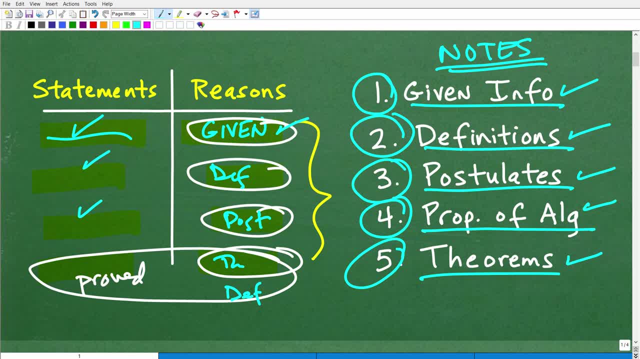 good answer. So I'm going to show you some examples of some of these things, and the way I'm going to show you some of these things is just to give some opinions. You've got to back it up with these things right here, okay. 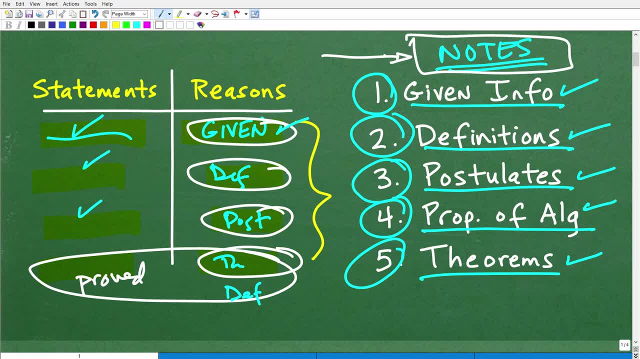 So, therefore, you better have super great notes, okay, Or this is going to become very difficult, and that's why a lot of students don't like doing these proms, because you know there's no way you're just going to be able to remember all this stuff. 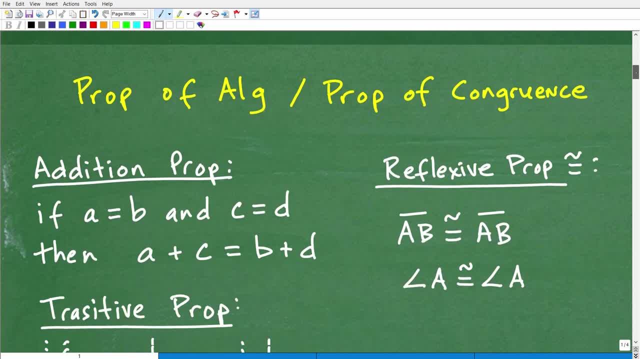 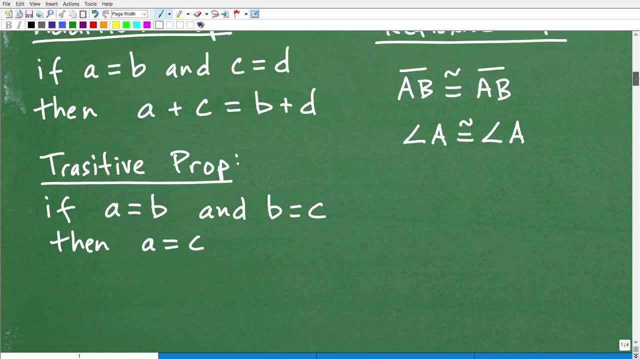 Okay, so let's go ahead and take a look at some examples of properties of algebra and congruence. So what am I talking about? Well, here's just a couple of quick examples, these things, But let's go ahead and take a look at a few. Okay, so you're probably saying, oh, 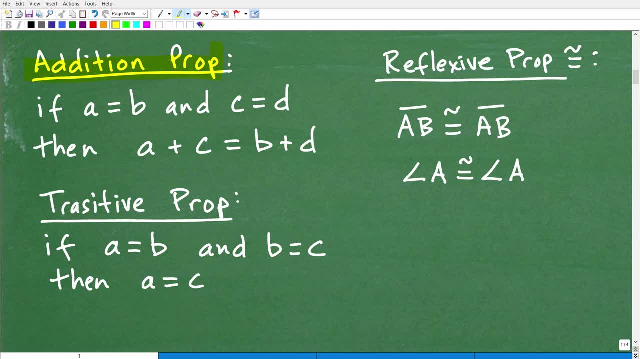 I remember learning this kind of stuff. Well, let's take a look at the addition property of algebra. Okay, now you can just kind of abbreviate this addition property. But let's take a look at this: If a equals b and c equals d, then a plus c is equal to b plus d. Now this seems like very 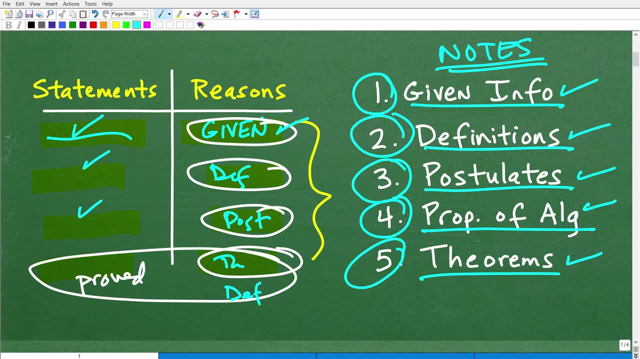 definitive answer to that. If you're not sure what it is, you're probably not going to be able to do a good enough job of answering it, but that's probably a good enough way to answer it, In other words, if there's a big difference between the two of them. 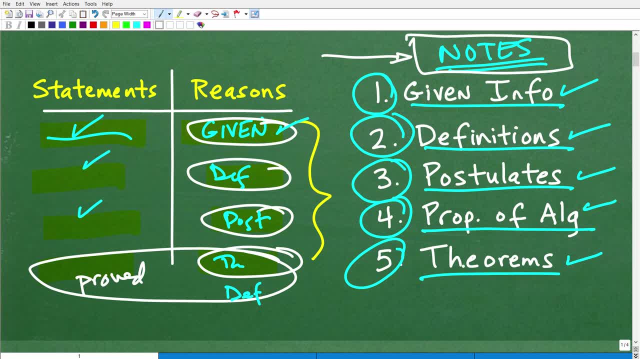 then you need to ask yourself: okay, these things are synonyms, these things are111 and they're pretty similar anyway. the other thing is they're not identifiable because they're just flaws in some of these things. and if you're going to bit by few of these things, 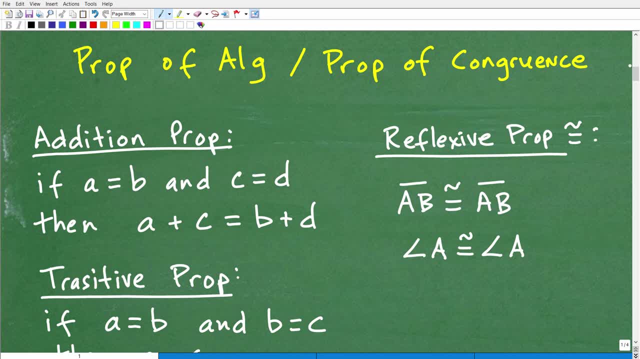 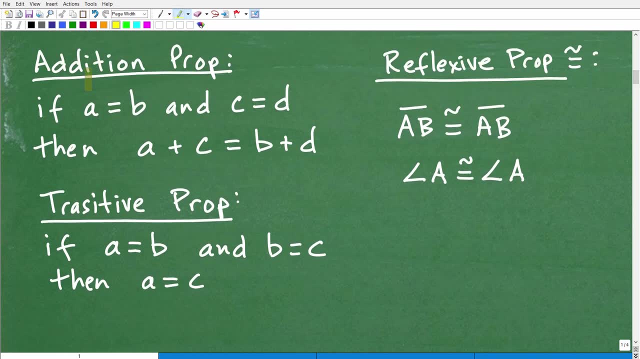 you actually need to give a little bit more of an answer to that one. So there's a lot of these things, these things, but let's go ahead and take a look at a few, okay. so you probably say, oh, I remember learning this kind of stuff. well, let's take a look at the addition property of algebra. okay. 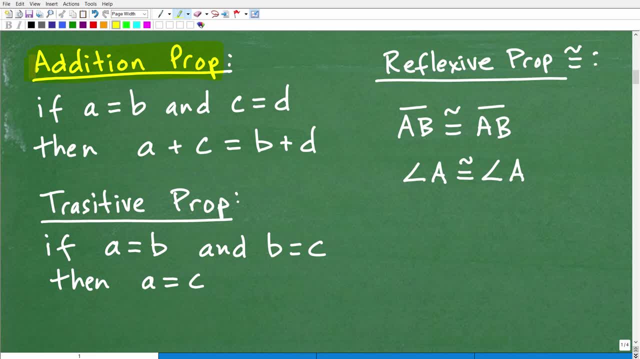 now you can just kind of abbreviate this addition property. but let's take a look at this: if a equals b and c equals d, then a plus c is equal to b plus d. now this seems like very obvious, right? look, if this is equal to this, okay, a is equal to b. well then. if c is equal to d, well, if I add c over here. 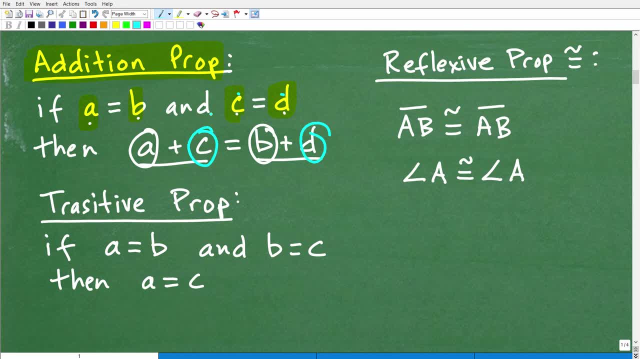 a plus c, that's the same thing as b plus d. okay, if you kind of study this for a second, it would seem like logical, right. you'll be like, yeah, you know, yeah, if a equals b and c equals d, then of course a plus c would equal to b plus d. but we need this right here has to be justified, okay, you. 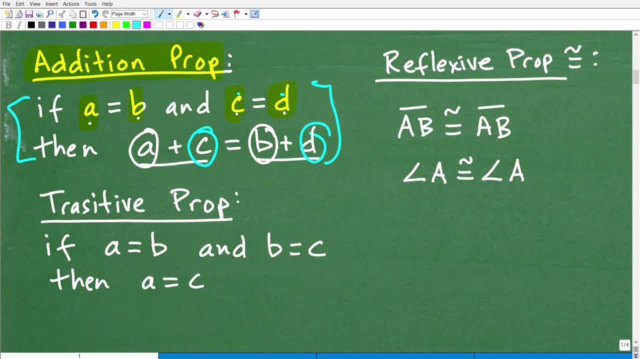 have to back this up formally. you have to back this up formally. you have to back this up formally. okay, so you have. you'd have to say: yes, this is true because of the addition property of algebra. okay, you just can't write this down. you have to actually know the name. okay, so it is important. 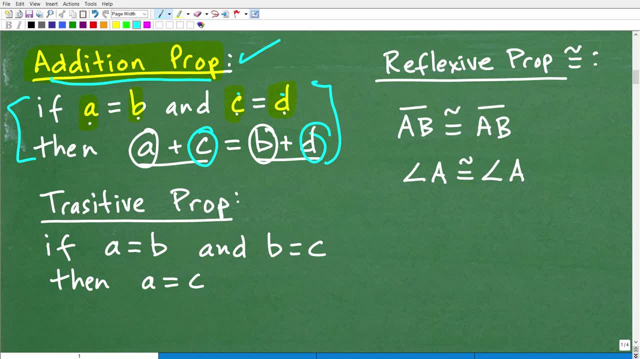 that you can identify these properties, definitions, etc. by name, and there's no way you're going to be able to remember all, remember all this stuff you got to reference your notes, okay, all right. so let's take a look at another example of another property example in algebra, and this is the. 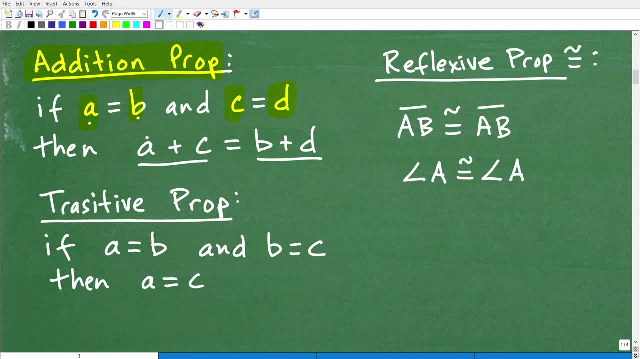 obvious, right? Look, if this is equal to this, okay, a is equal to b. Well then, if c is equal to d, well, if I add c over here, a plus c, that's the same thing as b plus d. Okay, if you kind of. 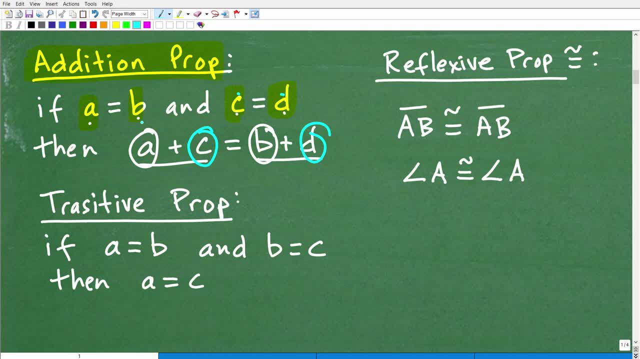 study this for a second. it would seem like logical right? You'll be like: yeah, you know, yeah, if a equals b and c equals d, then of course a plus c would equal to b plus d. But we need. 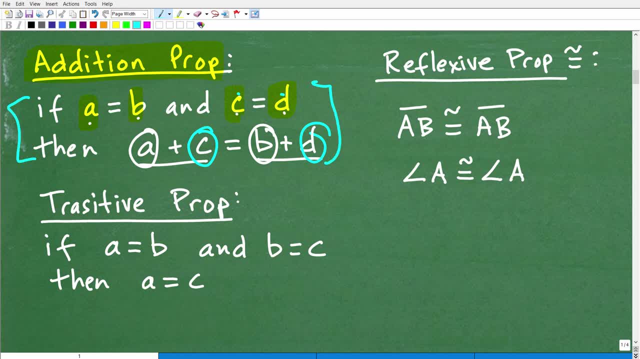 this right here has to be justified. Okay, you have to backtrack this up formally. Okay, so you'd have to say, yes, this is true because of the addition property of algebra. Okay, you just can't write this down. you have to actually know the name. Okay, So it is. 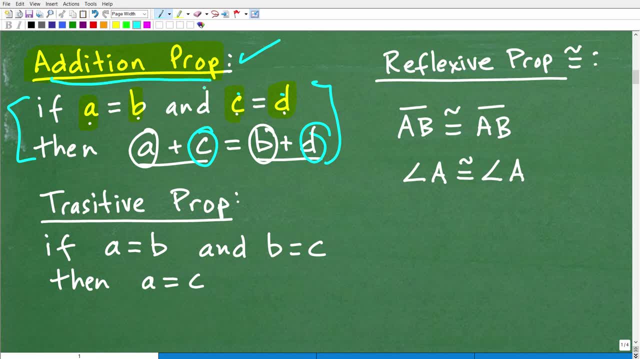 important that you can identify these properties, definitions, etc. by name, And there's no way you're going to be able to remember, remember all this stuff you got to reference your notes. Okay, All right. So let's take a look at another example of another property, example in algebra, And this: 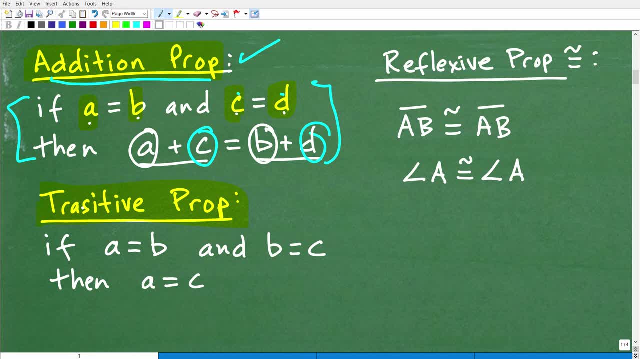 is the transitive property. I'm missing a little n here: transitive property. So the transitive property, big property. So here is the transitive property. If a equals b and b equals c, then a equals c Makes sense, right. If 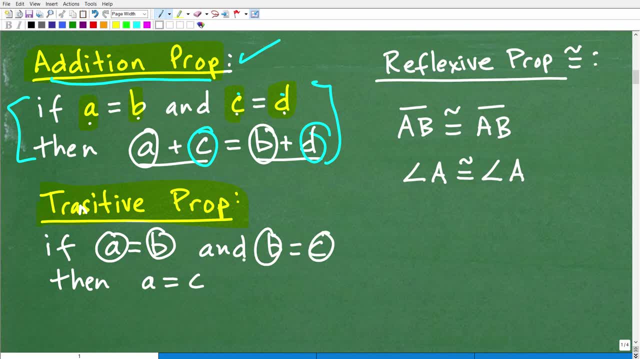 a equals b and then b equals c. All right, so I'm like: okay, a, b. So you can almost think of it this way: a equals b and then b equals c. Therefore, a is equal to c. It's totally. 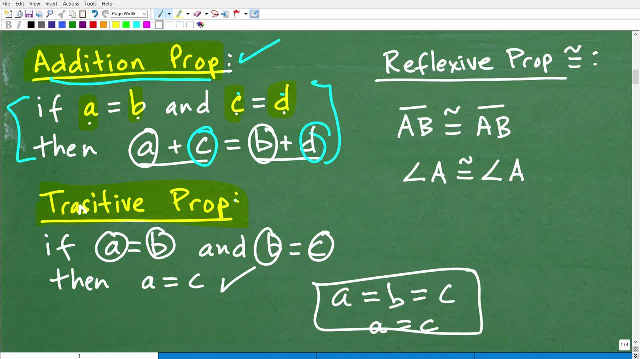 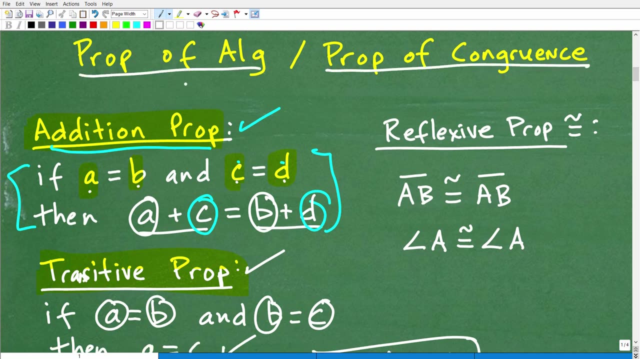 logical. Well, you got to back this up. This right here is true because it's something called the transitive property of algebra. Okay, Now let's go over here and take a look at congruence. There's also properties of congruence. Now, properties of algebra. you're typically going 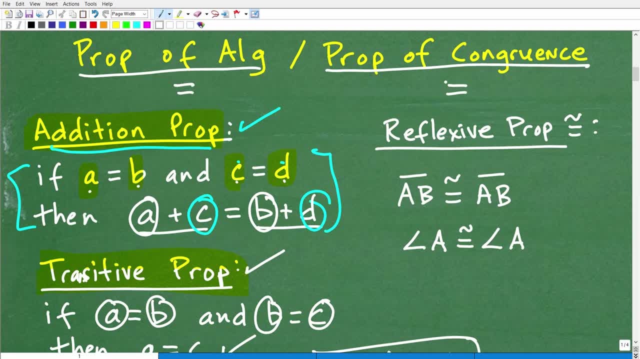 to have like an equal sign over here with properties of congruence. We're talking about this little congruent symbol right there. So what is congruence? Well, congruence here if I said, like the number two is equal to two, okay, that is just like a property of algebra. 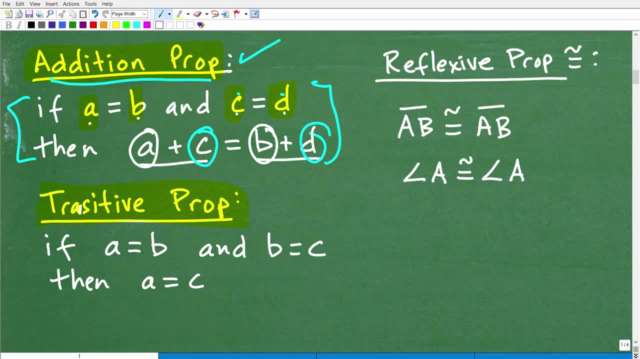 transitive property. I'm missing a little n here: transitive property. so the transitive property, big property. so here is the transitive property. if a equals b and b equals c, then a equals c. it makes sense, right? if a equals b and then b equals c, all right. so I'm like: okay, a, b, so you can almost think of it this way: a. 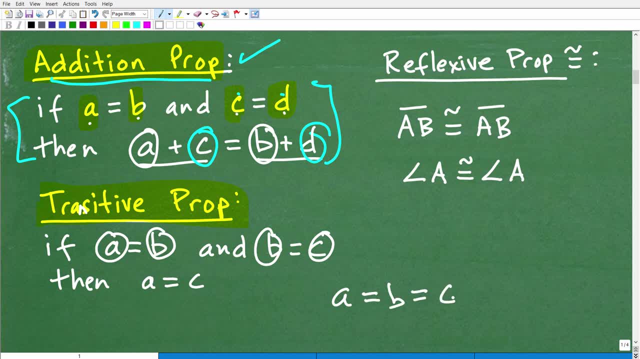 equals b, and then b equals c. therefore, a is equal to c. it's totally logical. well, you got to back this up this right here is true because of something called the transitive property of algebra. okay, now let's go over here and take a look at congruence. there's also properties of congruence. 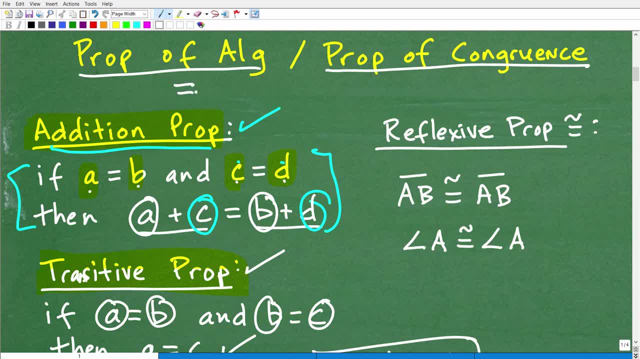 now properties of algebra. you're typically going to have like an equal sign over here with properties of congruence. we're talking about this little congruent symbol right there. so what is congruence? well, congruence here if I said, like, the number two is equal to two, okay, that is just like a property of algebra. okay, that would be like the. 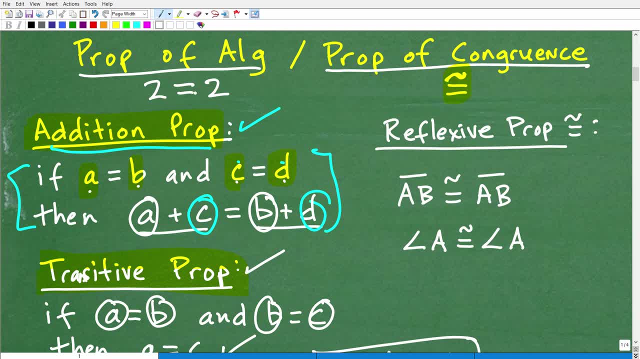 reflexive property. now we have a similar property. okay, it's basically the same property, but we call it the property of congruence. but congruence has to deal with measure, the measurement of, like, something that's given us a measure. okay, ie, let's actually take a look at an example. so let's. 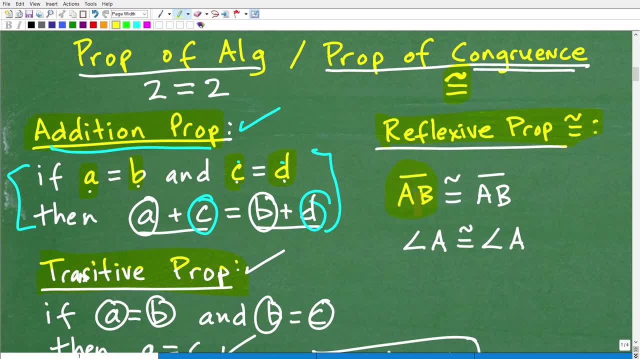 look at the reflective property of congruence, so line segment a- b is congruent to line segment a- b. in other words, here's a- b, it's basically the same measure of itself. okay, well, we can uh state that because of the reflexive property of 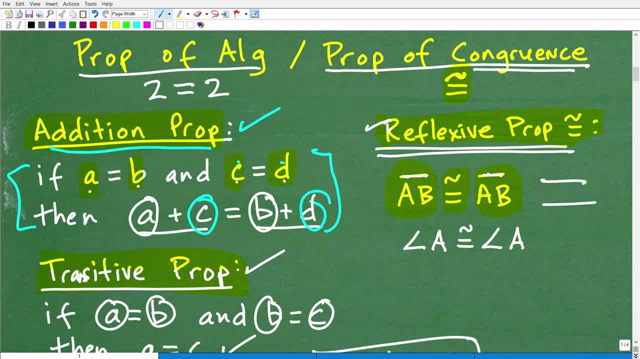 congruence because we're dealing with line segments. okay, we're actually measuring something. so when you're measuring line segments or angles, like here's another example- the reflexive property of congruence- angle a is congruent to angle a. so this would not be the reflexive property of algebra, to be more technical about it. you want to. 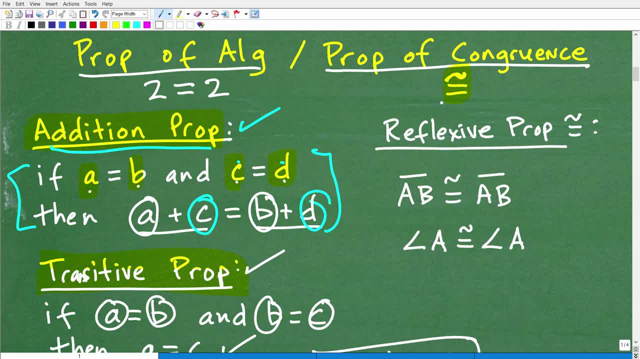 Okay, that would be like the reflexive property. Now we have a similar property. Okay, it's basically the same property, but we call it the property of congruence. But congruence has to deal with the measurement of, like, something that's given us a measure. Okay, ie, let's actually. 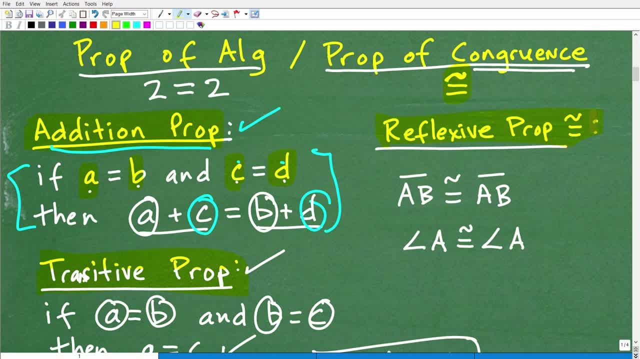 take a look at an example. So let's look at the reflective property of congruence. So line segment AB is congruent to line segment AB. In other words, here's AB, it's basically the same measure of itself. Okay, well, we can state that because of the 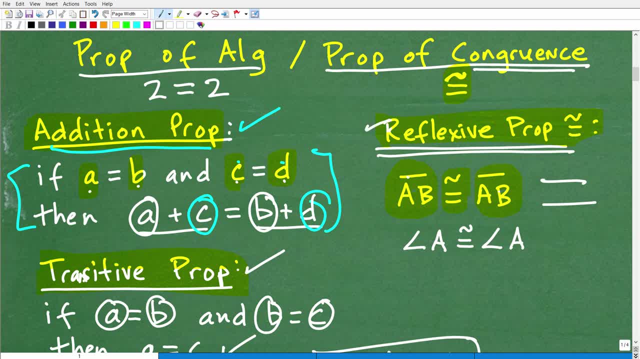 reflexive property of congruence, because we're dealing with line segments. okay, we're actually measuring something. So when you're measuring line segments or angles like, here's another example of the reflexive property of congruence: Angle A. 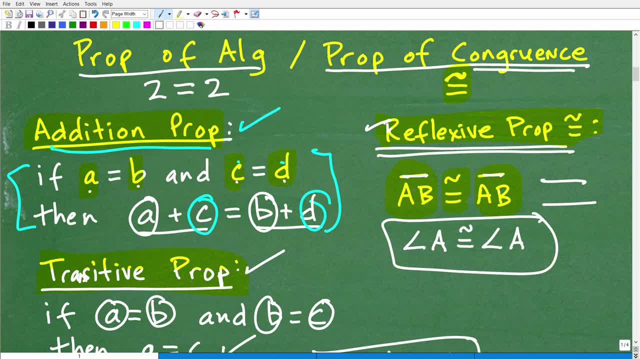 it's congruent to angle A. So this would not be the reflexive property of algebra. To be more technical about it, you want to have the reflexive property of congruence, But if I just said two is equal to two, that would just be the reflexive property. That's a property of algebra, So going 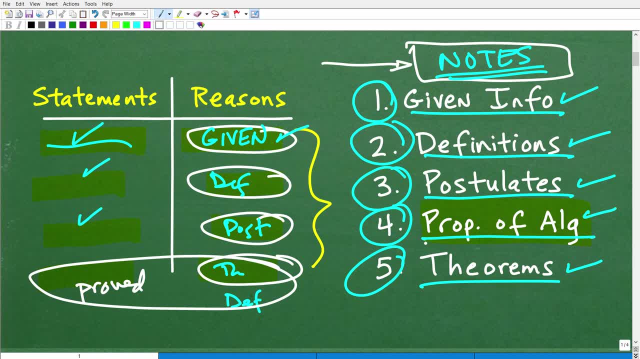 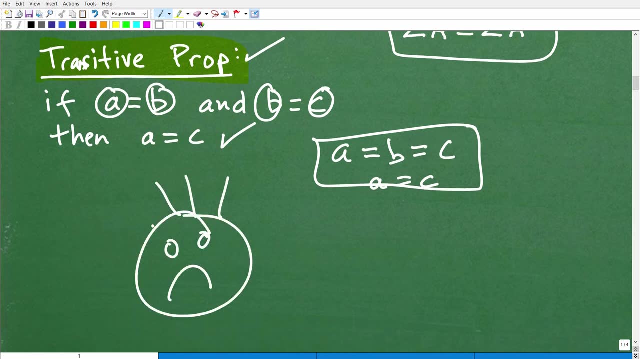 up here. okay, there are quite a few properties of algebra and congruence. They should be somewhere in your notes. Now. a lot of you are probably kind of flabbergasted at this level, but if you're, you might be going like this here, just like this is why I hate doing these problems, You know. 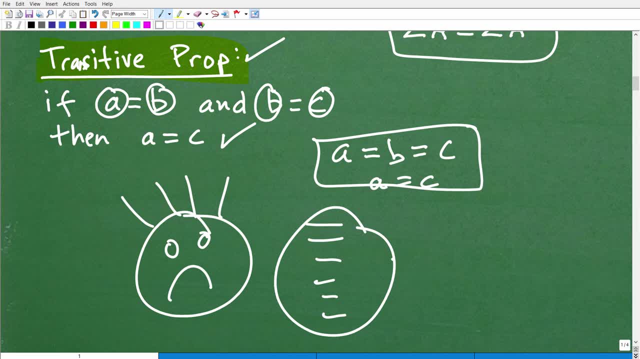 there's so much to know, just like. and then I got to, like, figure out how to actually do these things. Well, listen, don't give up the ship just yet. Okay, I'm trying to tell you what you need to work on in order to be organized. Okay, And in geometry, when you're dealing with proofs. 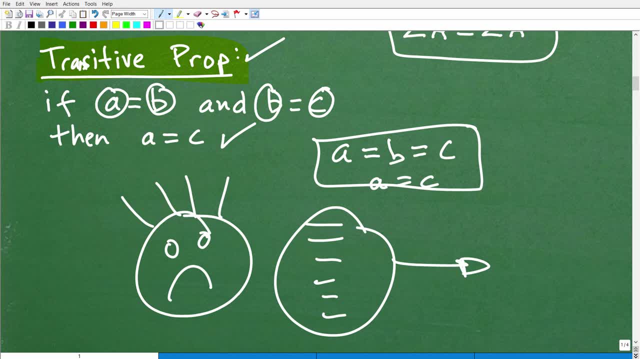 you're not going to. you know, really, you know be effective at this unless you can reference all of them. But listen, if your notes aren't where they need to be, just improve them. You can definitely go back and get yourself, you know, up to where you need to be. Okay, It's just going to. 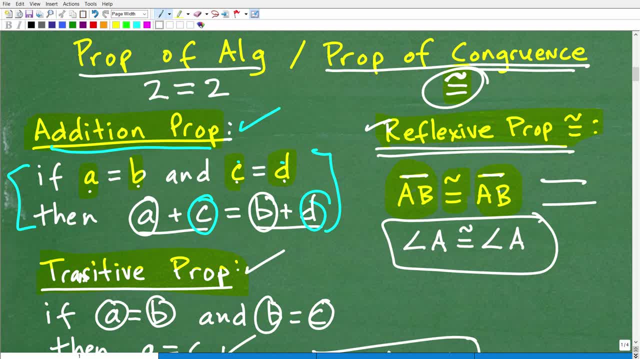 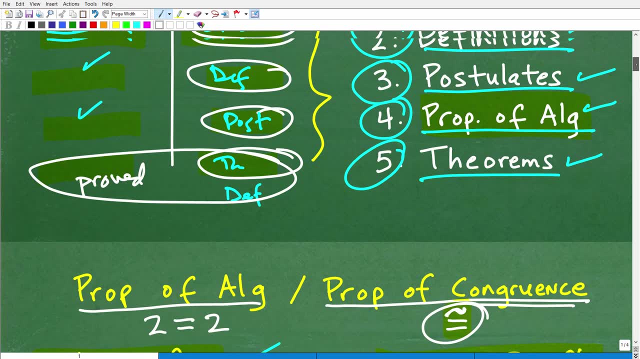 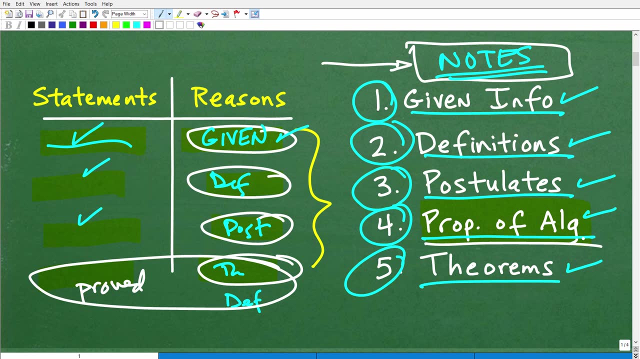 have the reflexive property of congruence. but if I just said two is equal to two, that would just be the reflexive property. that's a property of algebra. so going up here, okay, there are quite a few of properties of algebra and congruence. they should be somewhere in your notes now. a lot of you. 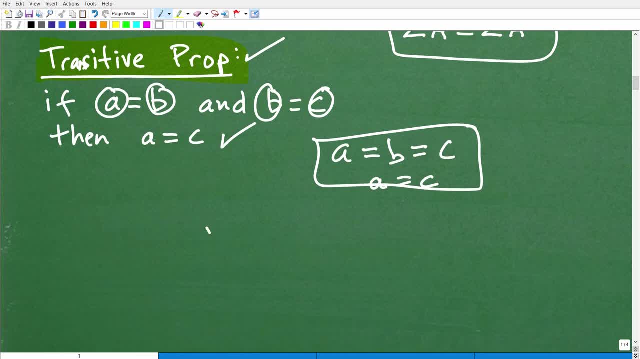 are probably kind of flabbergasted at this level. you might be going like this and you're going to do this. you're just like. this is why I hate doing these problems. you know there's so much to know, just like. and then I gotta like figure out how to actually do these things. well, listen, don't give up. 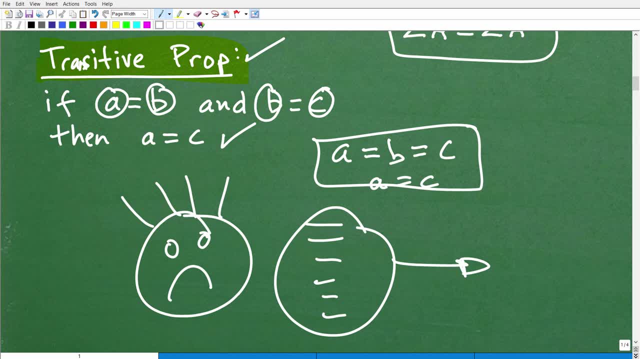 the ship just yet. okay, I'm trying to, um, tell you what you need to work on in order to be organized. okay, and in geometry, when you're dealing with proofs, you're not gonna, you know, really, uh, you know- be effective at this unless you can reference all this stuff. but listen, if your notes aren't. 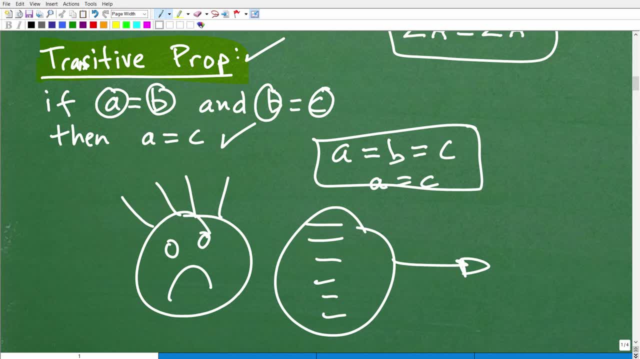 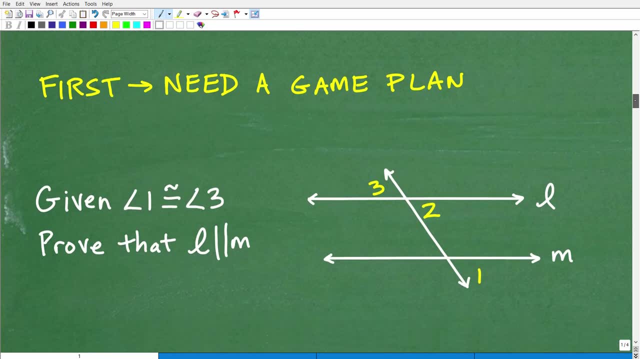 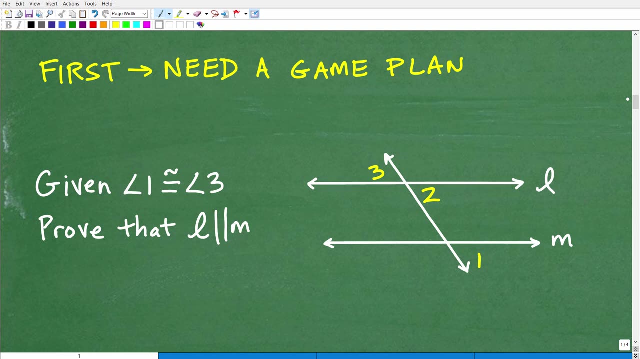 okay, just improve them. you can definitely go back and get yourself, you know, up to where you need to be. okay, it's just going to require a little bit of work. all right now. here comes the fun part. okay, so after we have a sense of that, we're going to be doing a two column proof. we know our reasons. 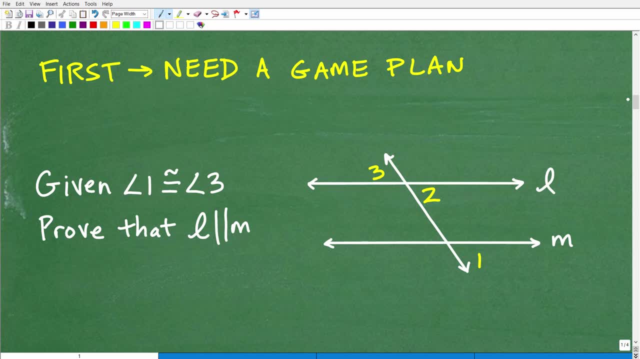 that we can give. okay, we kind of went over some examples of properties of algebra and properties of congruence. well, all of that, okay, is just the tools. okay, now we need to get creative and really our first move here those are kind of the rules of the game, but the game itself. 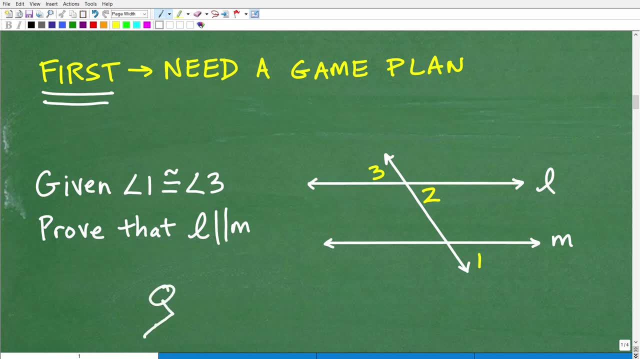 in order to prove something right. if you're gonna like, you know, here's you and here's your brother or sister and you guys are having an argument over something. now the game is: hey, I gotta convince this person that I'm right and they're wrong. okay, that's the game. so now that we know the rules, we 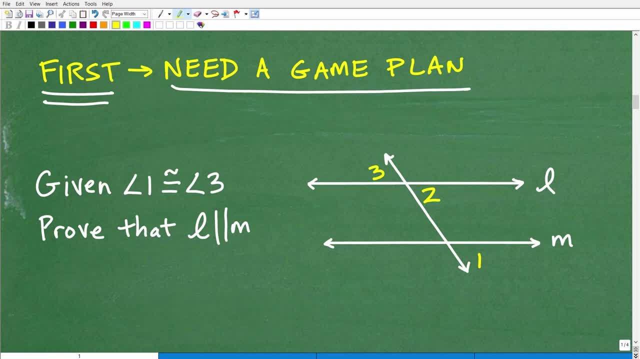 can prove this. so this is where it becomes fun, okay? so let's take a look at the situation here and we're saying, okay, given angle one is congruent to angle three. we've got to understand these words. so here's angle one and we're saying it's congruent to angle three. in other words this: 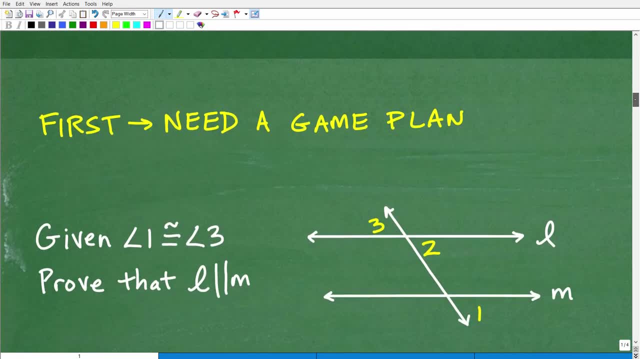 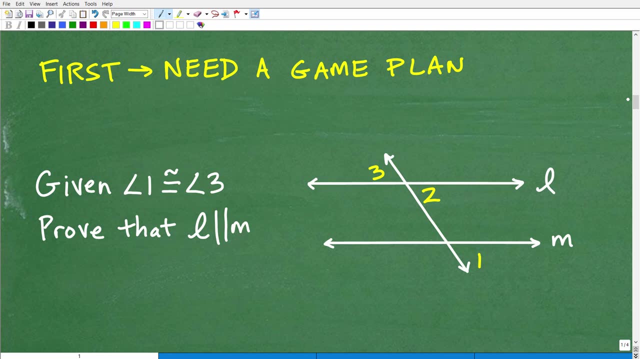 require a little bit of work. All right, Now here comes the fun part. Okay, So after we have a sense of that we're going to be doing a two column proof. We know our reasons that we can give. Okay, We kind of went over some examples of properties of algebra and properties of congruence. Well, 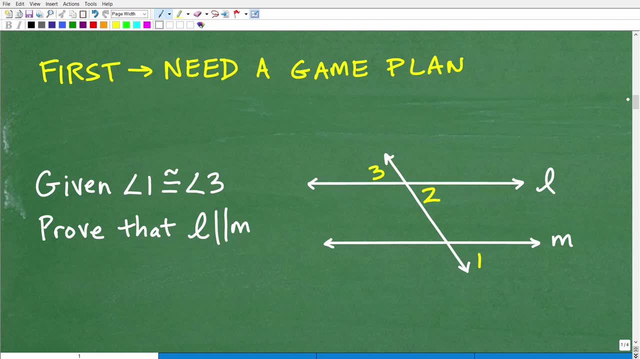 all of that okay is just the tools. Okay. Now we need to get creative And really our first move here, those are kind of the rules of the game, but the game itself, in order to prove something right, If you're going to like. 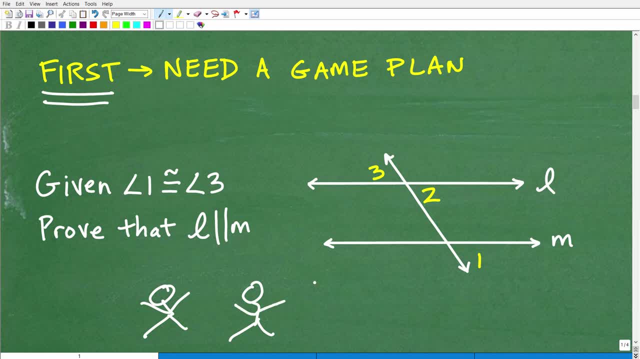 you know, here's you and here's your brother or sister, and you guys are having an argument over something. Now the game is: Hey, I got to convince this person that I'm right and they're wrong. Okay, That's the game. So now that we know the rules, we need a game plan to uh. 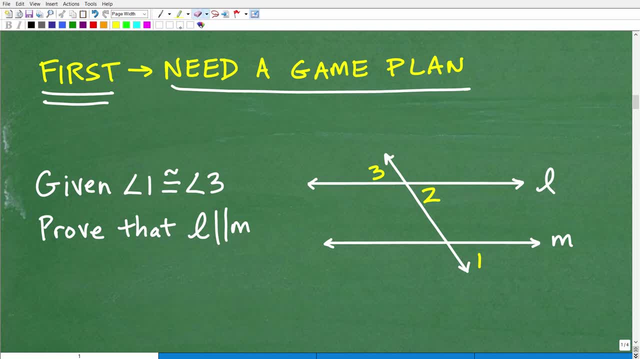 prove our point. Okay, So this word, this is where it becomes fun. Okay, So let's take a look at the situation here. And we're saying, okay, given angle one is congruent to angle three. We've got to understand these words. So here's angle one And we're saying it's congruent to. 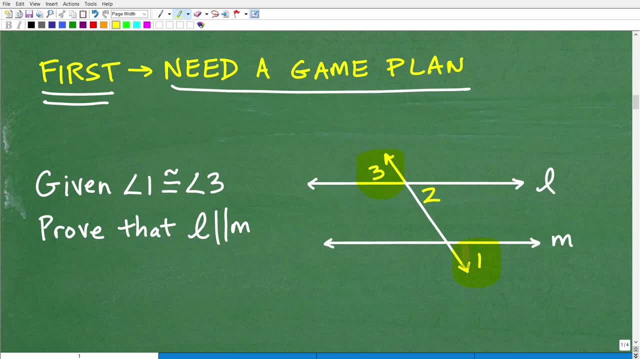 angle three. In other words, this angle and this angle are equal. We're like: okay, All right, That's given to me. I want to prove that these two lines are parallel. Okay, So it's probably going to help us to review a lot of theorems and postulates about parallel lines. So 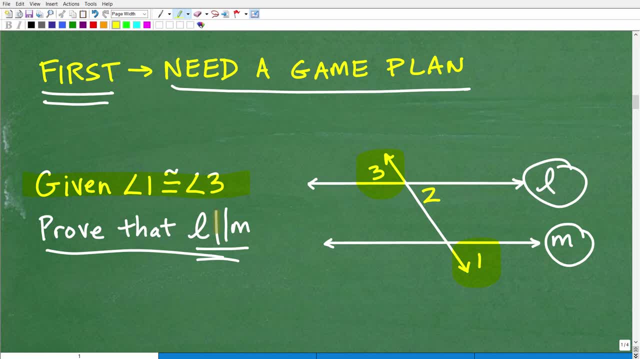 this is the key. Okay, This proof has to do with, uh, proving two lines are parallel. So what you want to be thinking- and your little thinking cap there is, you're going to be saying to yourself: okay, what do I know about parallel lines? So you need to be thinking about all the theorems. 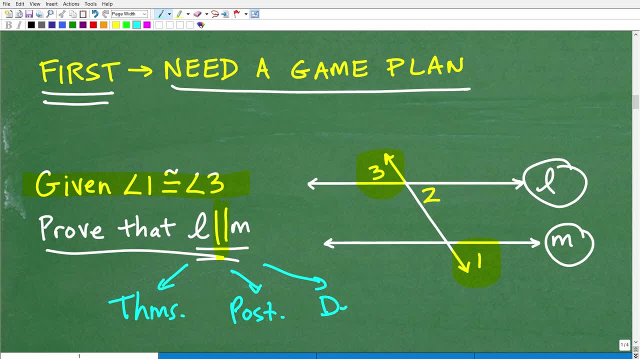 you know all the postulates, you know, and, like the definition of parallel lines, you got to be thinking, okay, what do I have? Okay, And this is all. this stuff should be in your notes. Okay, Now we want to be. 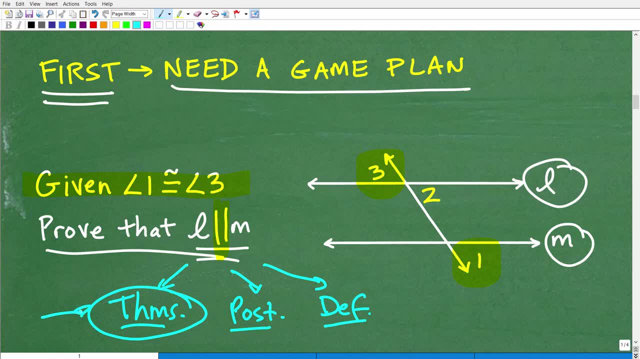 thinking about in this particular problem, uh, a certain theorem that can help us out. but I'm kind of jumping the gun here, So you're like, all right, I know a lot about parallel lines and I, uh, I'm seeing that two and angle one, these two angles here, Okay, Cause I didn't in. 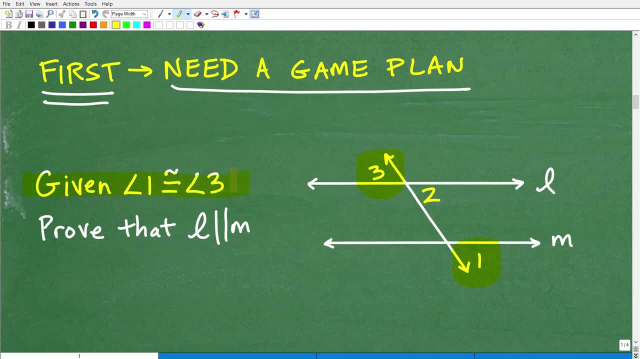 angle and this angle are equal, we're like: okay, all right, that's given to me. I want to prove that these two lines are parallel. okay, so it's probably going to help us to review a lot of theorems and postulates about parallel lines. so this is the key. okay, this proof. 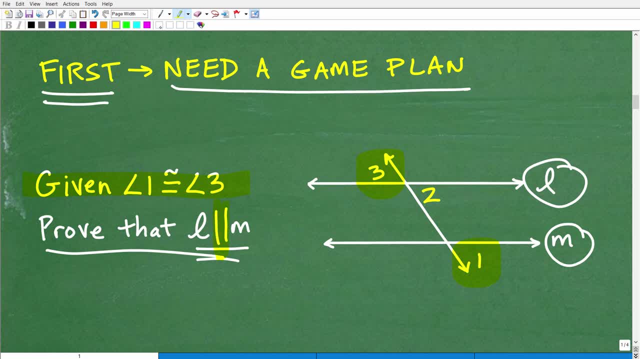 has to do with, uh, proving two lines are parallel. so what you want to be thinking in your little thinking cap there is you're going to be saying to yourself, okay, what do i know about parallel lines? so you need to be thinking about all the theorems you know, all the postulates, you know and, like the 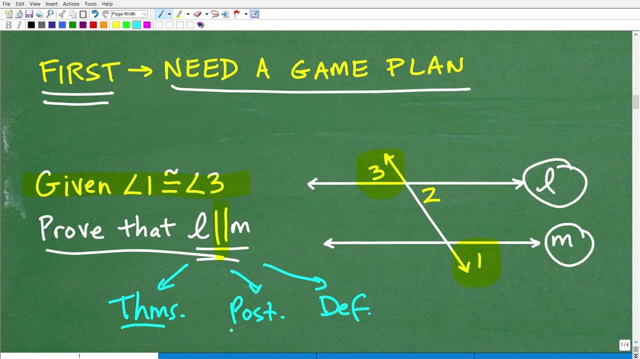 definition of parallel lines. you got to be thinking, okay, what do i have? okay, and this is all. this stuff should be in your notes. okay, now we want to be thinking about in this particular problem, uh, a certain theorem that can help us out. but i'm kind of jumping the gun here. 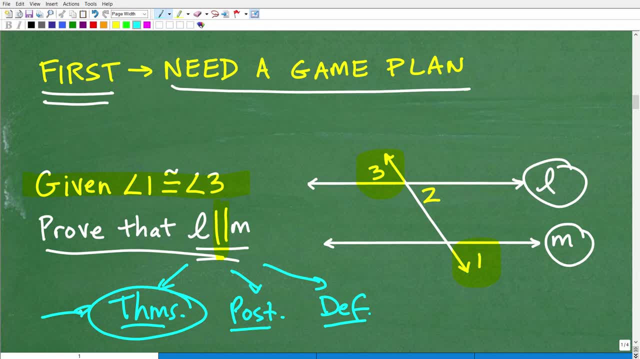 so you're like: all right, i know a lot about parallel lines and i i'm seeing that two in angle one, these two angles here? okay, because i didn't in the given information, angle two wasn't mentioned, but these two angles are what kind of angles? they're corresponding angles, okay, and there's 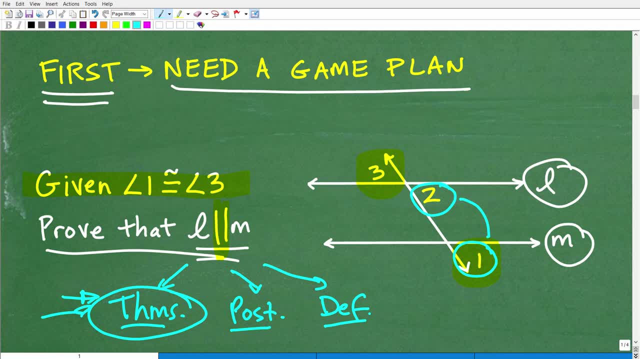 a theorem you're saying: oh, corresponding angle. wait a minute. i remember seeing a theorem that said: if two core corresponding angles formed by a transversal and two parallel lines, okay. if two corresponding angles form by a transversal and two lines, okay if these two corresponding angles. 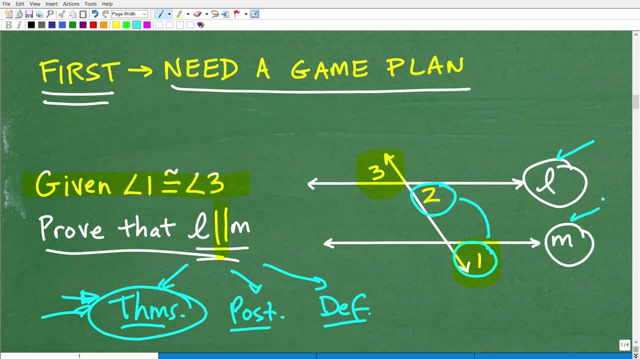 are congruent, then these lines are parallel. now i kind of just paraphrase that, but that's effectively what a theorem would look like now in your book or in your course. you might be like there, if you know, your teacher might have that as theorem one or whatever it's going to be categorized. but you're going to have some. 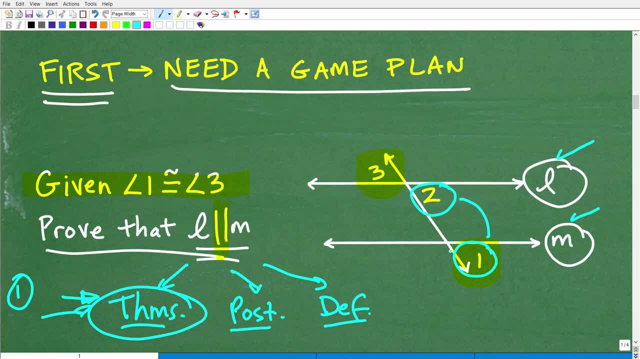 sort of theorem that you learn that says: hey, if you have a transversal and two lines and these corresponding angles here, okay, or corresponding angles are congruent, well, that is telling you that the lines here are indeed parallel. so that's what we want to shoot for. our game plan is like: oh, okay, so why don't we get um? 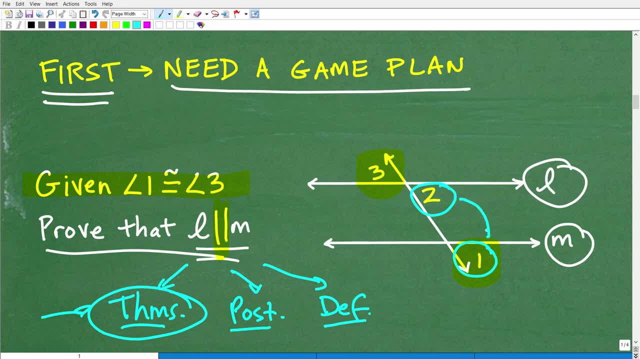 the given information. angle two wasn't mentioned. but these two angles are what kind of angles? they're corresponding angles, Okay, And there's a theorem you're saying, Oh, corresponding angle. Wait a minute. I remember seeing a theorem that said: if two core corresponding angles formed by a 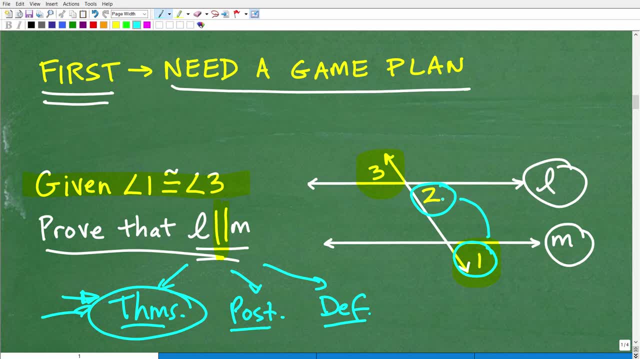 transversal and two parallel lines. Okay, If two corresponding angles formed by a transversal and, uh, two lines. Okay, If these two corresponding angles are congruent, then these lines are parallel. Now I kind of just paraphrase that: 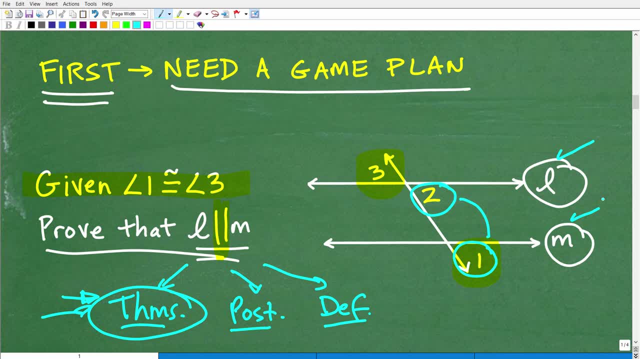 but that's effectively what a theorem would look like now in your book or in your course you might be like there, you know your teacher might have that as theorem one or whatever It's going to be categorized. but there you're going to have some sort of theorem. 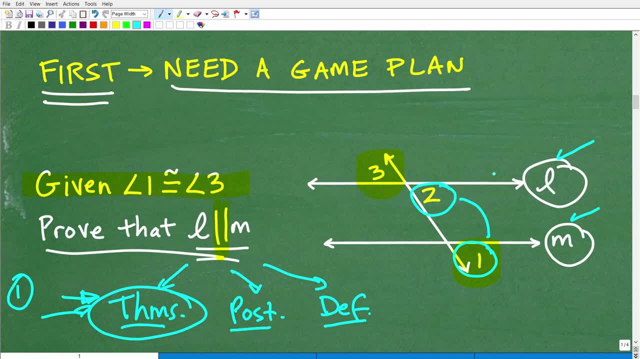 that you'll learn. that says: Hey, if you have a transversal and two lines and these corresponding angles here, okay, Or corresponding angles are congruent. Well, that is telling you that the that the lines here are indeed parallel. So that's what we want to shoot for. 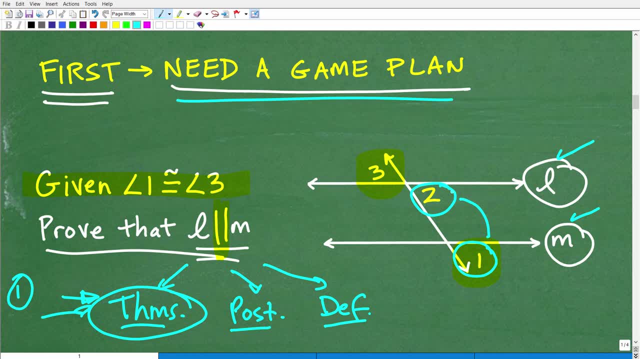 And it's like: Oh, okay, So why don't we get um, construct a plan to argue that angle two and angle one are corresponding? Now can we do that, Absolutely Okay, So we can say: hmm, angle three and angle two, All right, These two angles right, here are what we call. 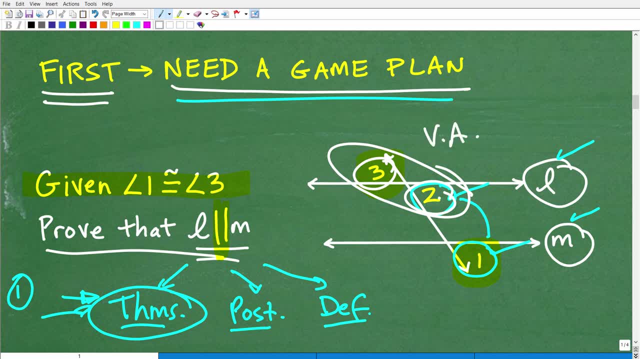 vertical angles. Okay, You're like: Oh yeah, vertical angles, These two angles are congruent, All right. In other words, they're the same, So this is the same as this. Okay, Three is the same as two and three. 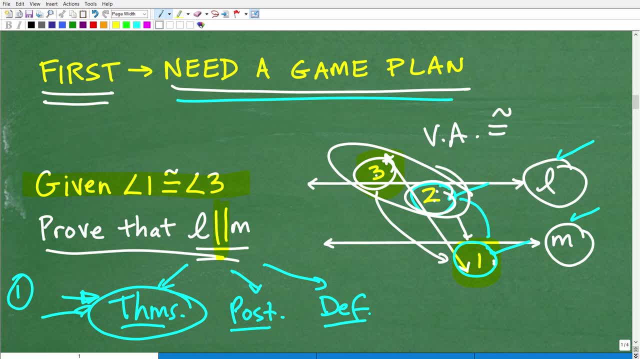 Three is the same as one, So therefore, two is the same as one. Okay, So I can say: okay, two is the same as one, And that's what I need. Okay, Two is the same as one, meaning that these corresponding angles are congruent. Therefore, I can make a final statement that 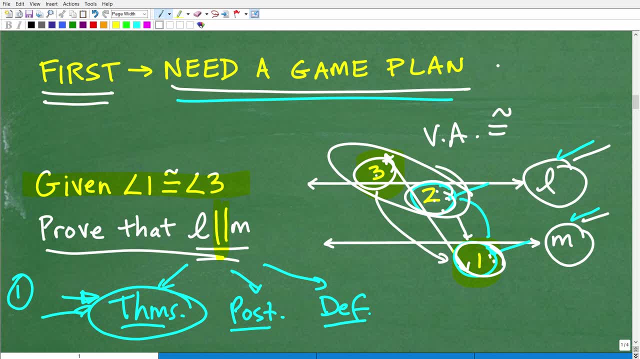 these two lines are parallel, So this is where the interesting part comes in. You need to kind of um a game plan. Don't start doing a proof until you construct this. Now, if you saw another strategy to get to this and maybe you're using another, you're using another strategy to get to. 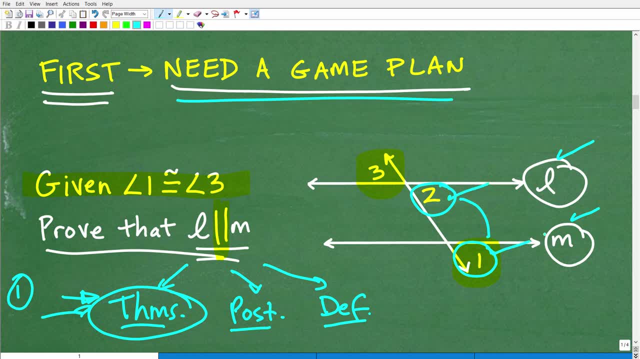 construct a plan to argue that angle two and angle one are corresponding. now can we do that? absolutely okay, so we can say: hmm, angle three and angle two, all right, these two angles right here are what we call vertical angles. okay, you're like: oh yeah, vertical angles. 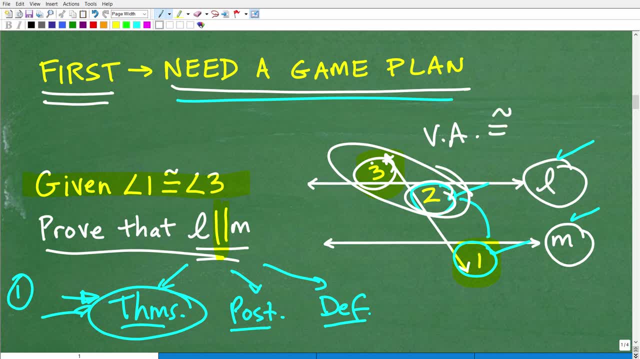 these two angles are congruent, right. in other words, they're the same. so this is the same as this. okay, three is the same as two and three is the same as one. so therefore, two is the same as one. okay, so i could say: okay, two is the same as one, and that's what i need. okay, two is. 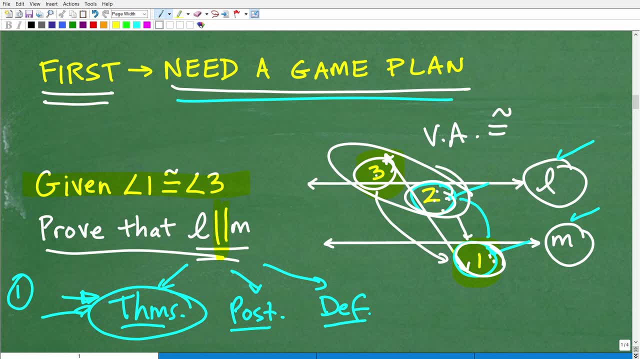 the same as one, meaning that these corresponding angles are congruent. therefore, i can make a final statement that these two lines are parallel. so this is where the interesting part comes in. you need to kind of um a game plan. don't start doing a proof until you construct this. 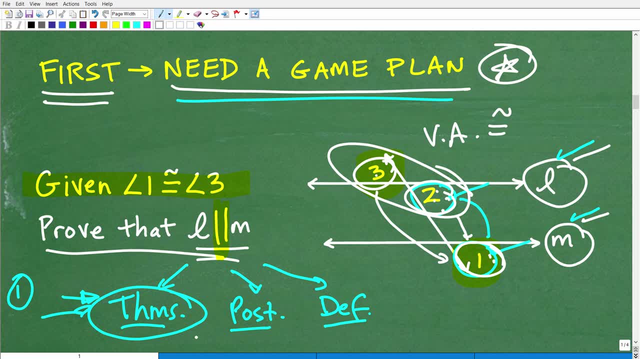 now, if you saw another strategy to get to this and maybe you're using another theorem or whatever the case is, there are other ways you can do this. okay, but you want to kind of look at the most elegant, uh, most effective, efficient way to prove your point. but that's okay, i mean, as long as you 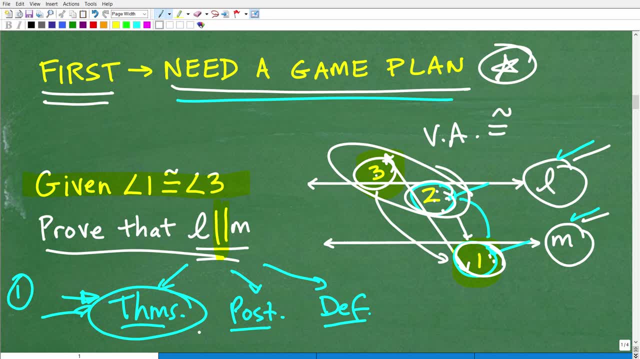 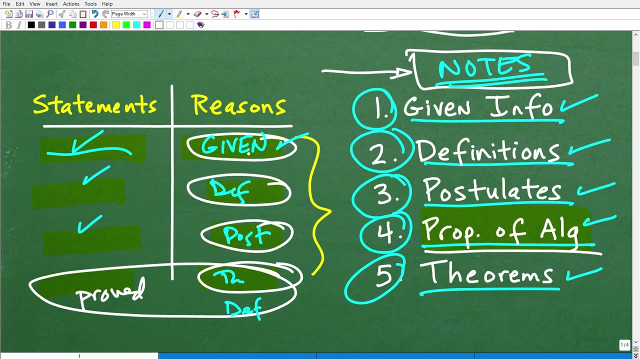 get it right. that's really the main, um, the main thing here. okay, all right. so, with that being said, if you want to try this on your own before you see my final answer, what you want to do now is make a statement, okay, which is typically going to be the given, and then you're going to use a definition postulate. 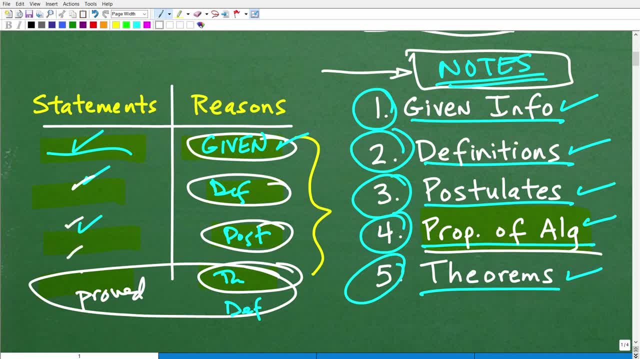 property of algebra, congruence or theorem, to kind of walk through. okay and uh, your final statement will be that um is your. your final statement is always going to be: line l is parallel to line m, in this particular case, because of your final reason. okay, so this is what you're going. 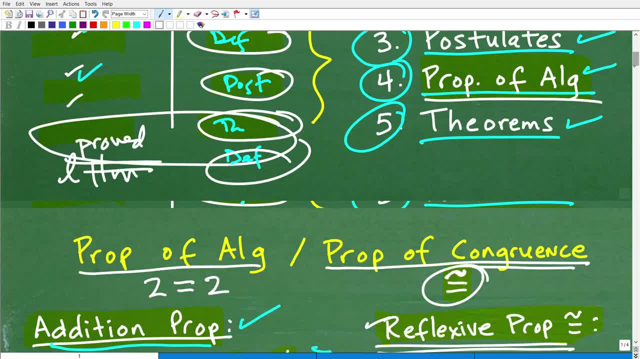 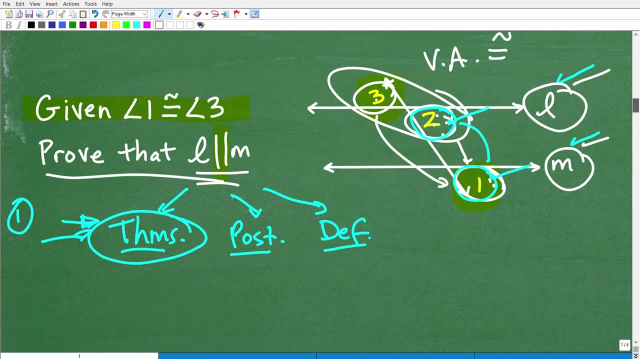 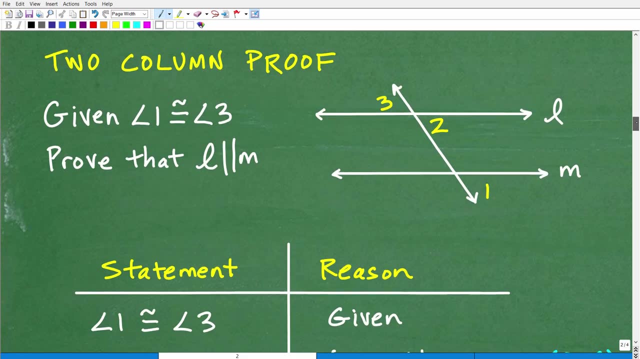 to think through. we have a game plan, so now we have to kind of tell that story. all right, so let's go down here and actually do this now. if you want to, you know, play around with this for a second, go to pause video and construct the proof, but let's go ahead and see my work again. you could. 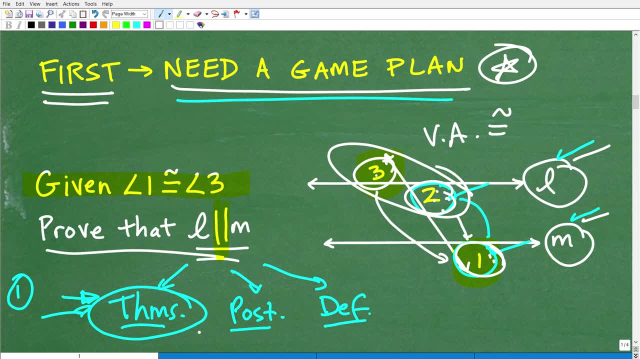 the theorem or whatever the case is. there are other ways you can do this. Okay, But you want to kind of look at the most elegant, uh, most effective, efficient way to prove your point. but that's okay, I mean, as long as you get it right. that's really the main um, the main thing. 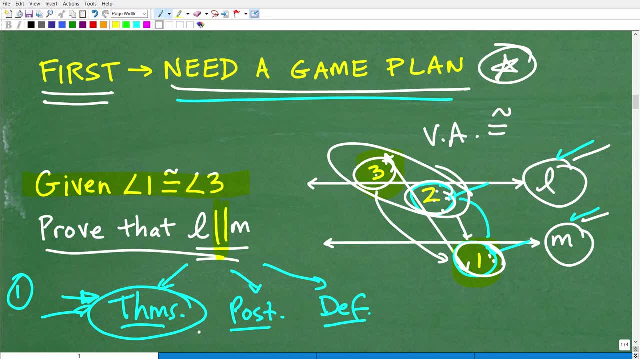 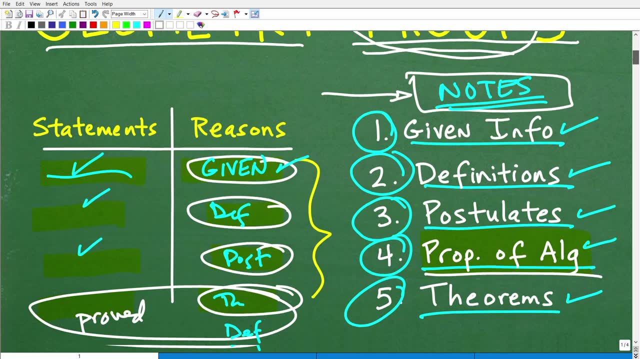 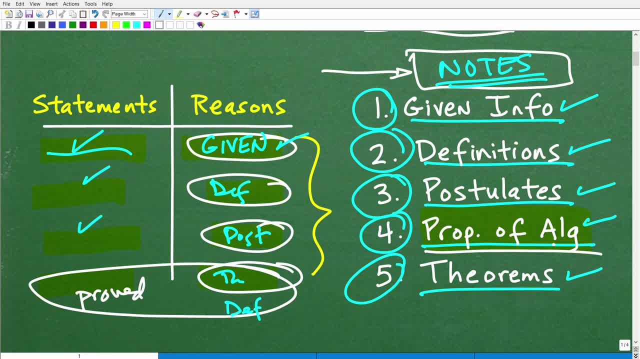 use a definition, postulate, property of algebra, congruence or theorem to kind of walk through Okay And uh. your final statement will be that um is your. your final statement is always going to be a: line L is parallel to line M in this particular case. because of your final reason. 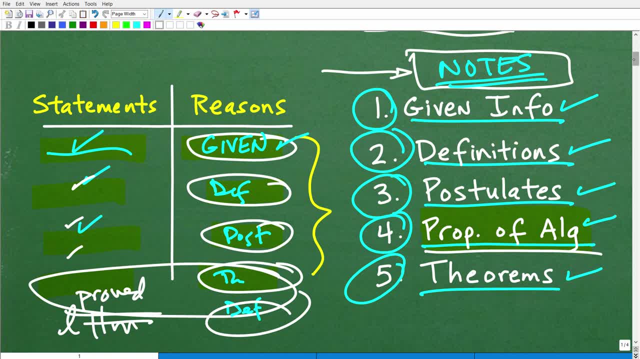 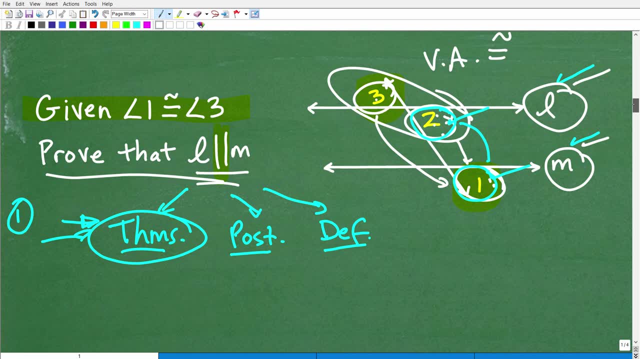 Okay, So this is what you're going to think through. We have a game plan, So now we have to kind of tell that story. All right, So let's go down here and actually do this Now. if you want to, you know, play around with this for a second- go ahead and pause the video and construct. 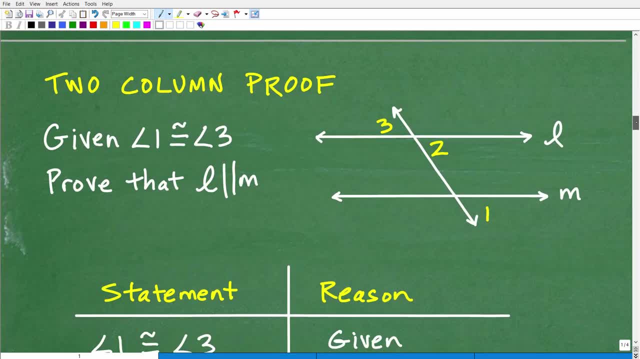 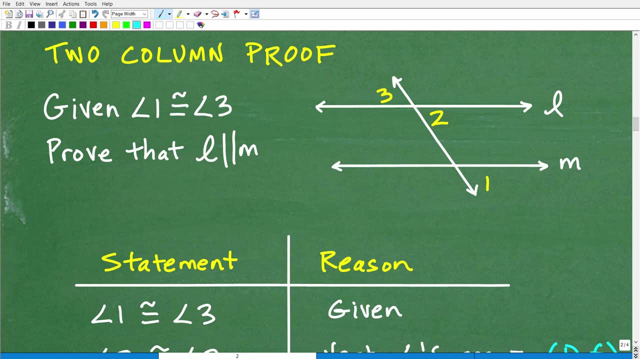 the proof. but let's go ahead and see my work Again. you could have done this, maybe a different way, but this is going to be the most uh direct route, uh to take. All right. So two column proof for this. So, given angle one is congruent to angle three, proven uh. line L is uh parallel. 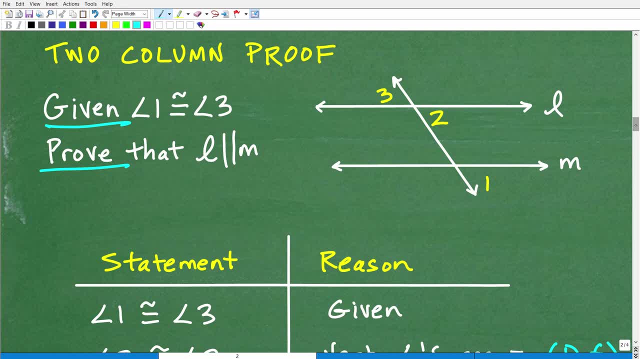 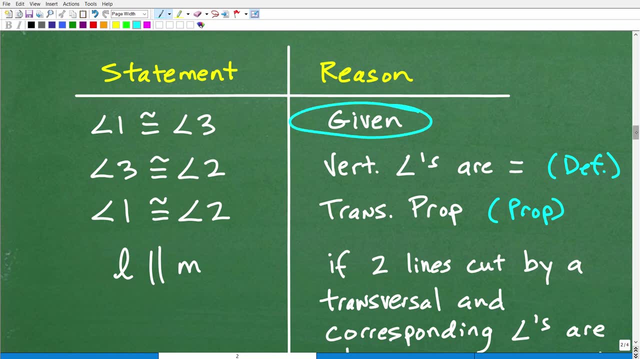 to line M. Of course that's the problem. Let's go ahead and get into it now. Okay, So angle one, that is given. all right, this is typically going to be your first uh move And then kind of think: 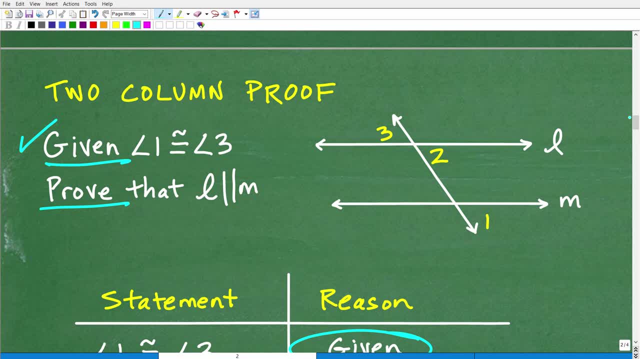 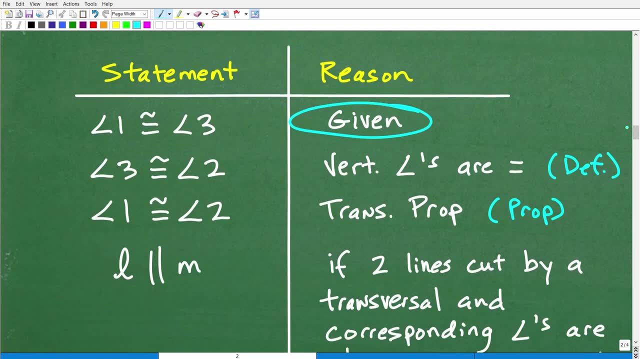 of this as playing a chess game or checkers game. You're like, okay, you're to make one move, And typically repeating the given information is almost always your first statement. So just get in the habit of just putting that down: Boom. So now I'm going to say angle three is congruent. 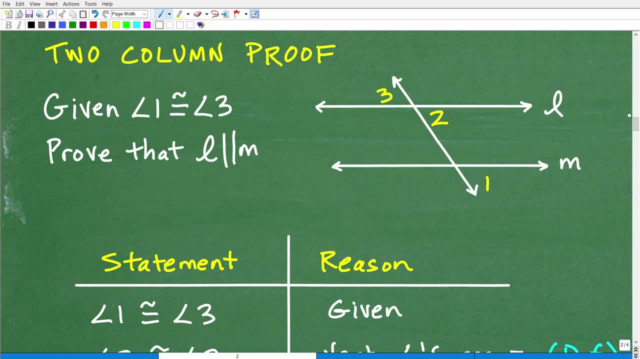 have done this maybe a different way, but this is going to be the most uh direct route, uh to take, all right. so two column proof for this. so, given angle one is congruent to angle three. proven line l is uh parallel to line m. of course, that's the problem. let's go ahead and get into it now. 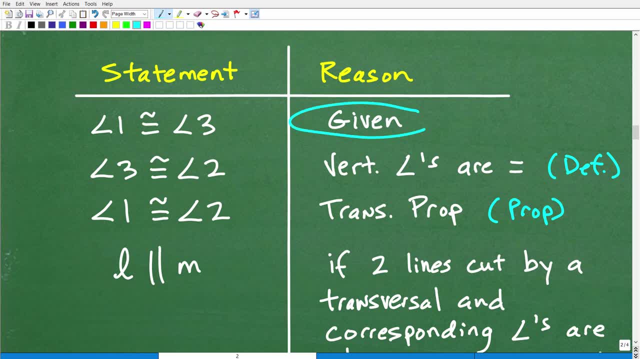 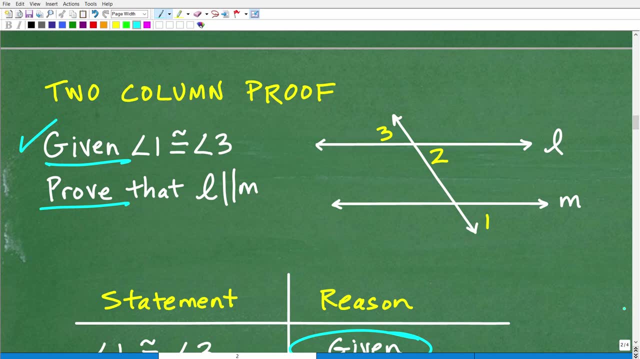 okay, so angle one is congruent to angle three. that is given. all right. this is typically going to be your first uh move and then kind of think of this as playing a chess game or checkers game. you're like, okay, you're to make one move and typically repeating the given information. 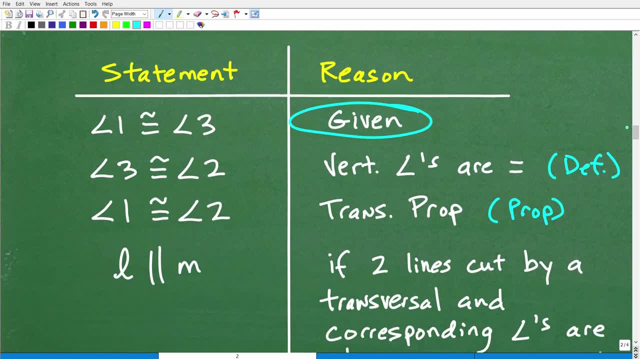 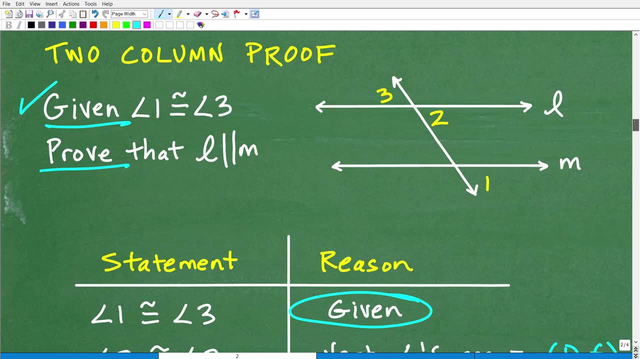 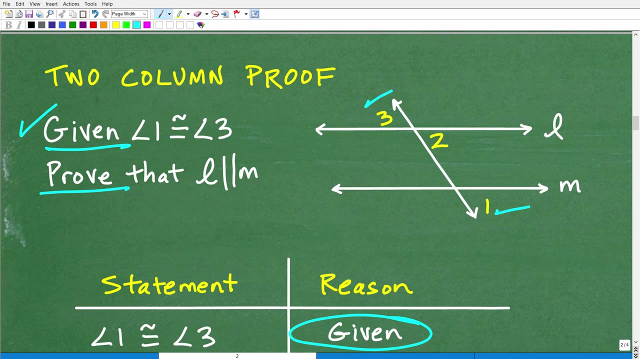 is almost always your first statement, so just get in the habit of just putting that down: boom. so now i'm going to say angle 3 is congruent to angle 2.. so remember, over here i'm already being told that 3 and 1 are the same angle. that's given information. but in order for me, 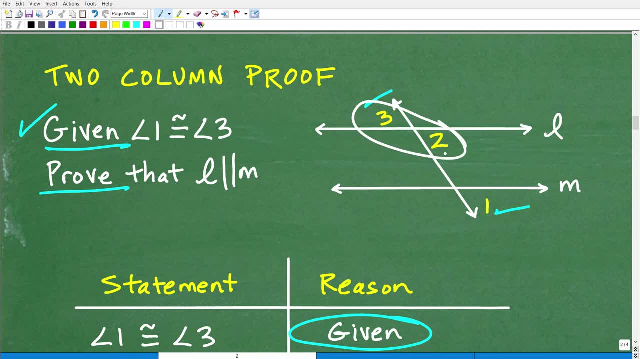 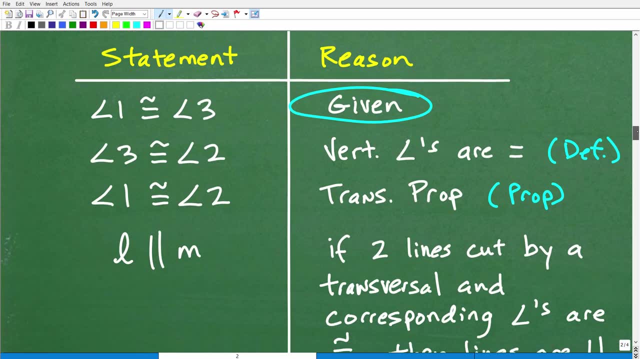 to make my little case here, i need to justify that 3 and 2 are the same. and 3 and 2 are the same because of vertical angles. so that's my next reason. i can't do anything until i make uh, establish, establish that back. so angle 3 is congruent to angle 2. why? because 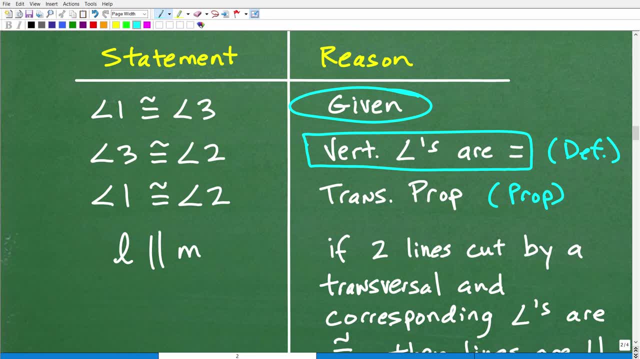 uh, vertical angles. okay, vertical angles are congruent, all right. three and two are vertical angles by definition, and vertical angles are congruent. so that is the definition of vertical angles. okay, all right. so there is somewhere along the lines you learned about vertical angles. that is a definition, okay, so now let's move on to our next uh statement. 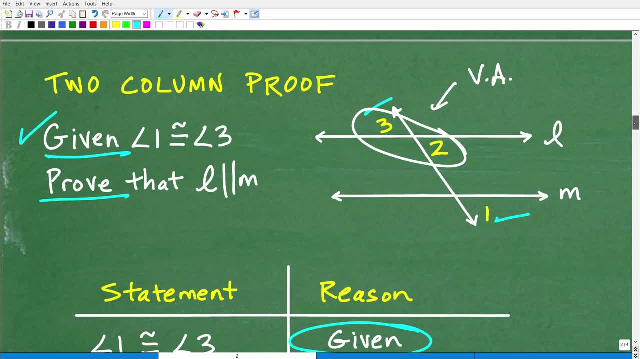 i'm going to say angle 1 is congruent to angle 2.. all right, so now that i made that, uh, point 3 is equal to 2. 3 is also equal to 1, so therefore, 2 is equal to 1.. remember, this is my next. 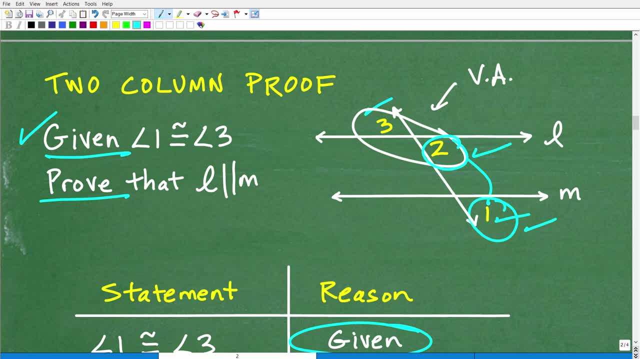 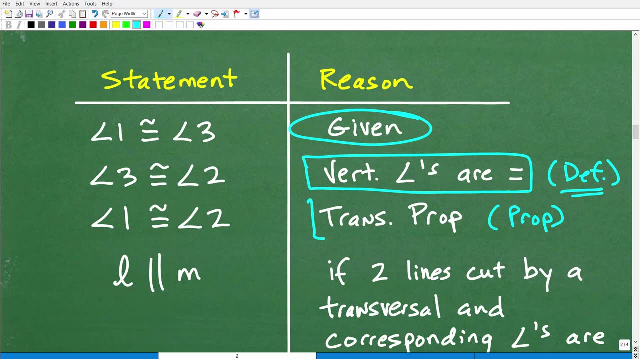 strategy. i want to show that these corresponding angles are equal, so let's go ahead and state that. but i got to back it up. so angle 1 is congruent to angle 2. why? because of the transitive property. okay, and to be more technically correct, you could put the transitive property of congruence. 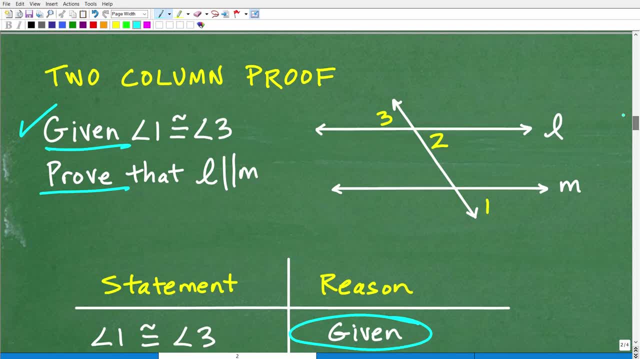 to angle two. So remember over here my um. I'm already being told that three and one are the same angle. that's given information. But in order for me to make my little case here, I need to justify that three and two are the same. and three and two are the same because of: 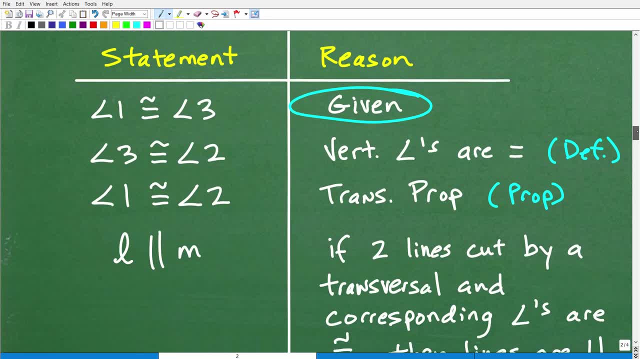 vertical angles. So that's my next reason. I can't do anything until I make uh establish. establish that back. So angle three is congruent to angle two. Why? Because, uh, vertical angles, okay, Vertical angles, are congruent, right. Three and two are vertical angles by definition. 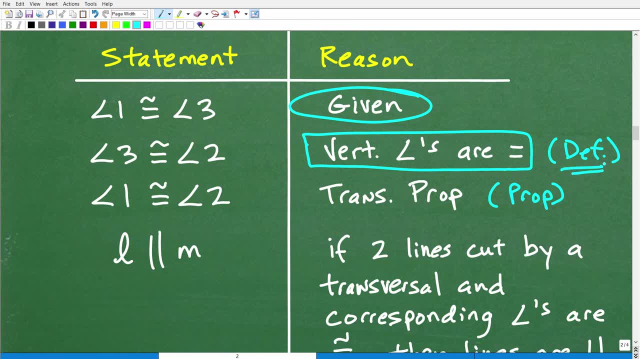 and vertical angles are congruent. So that is a definition of vertical angles. Okay, All right. So there is somewhere along the lines you learned about vertical angles. That is a definition, Okay. So now let's move on to our next statement. I'm going to say: angle one is congruent to angle two, All right. So now that I 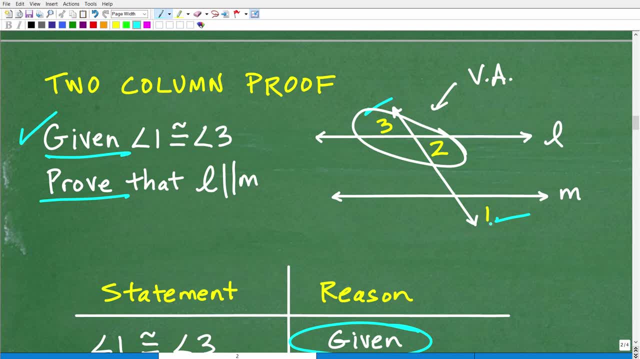 made that point. three is equal to two. three is also equal to one, So therefore two is equal to one. Remember, this is my next strategy. I want to show that these corresponding angles are equal. So let's go ahead and state that. but I got to back it up. So angle one is congruent to 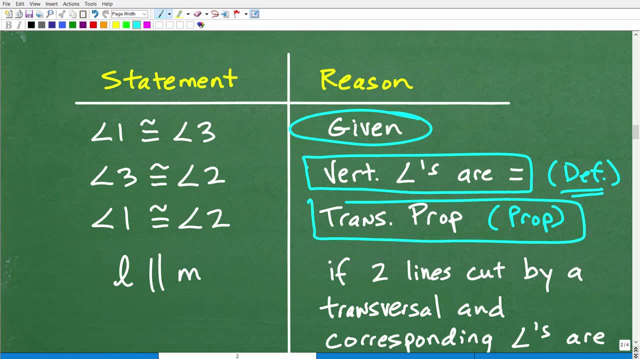 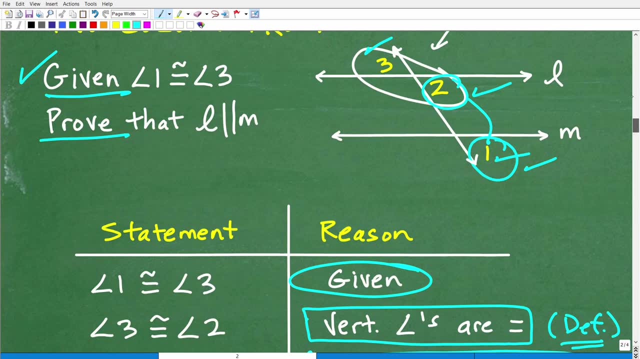 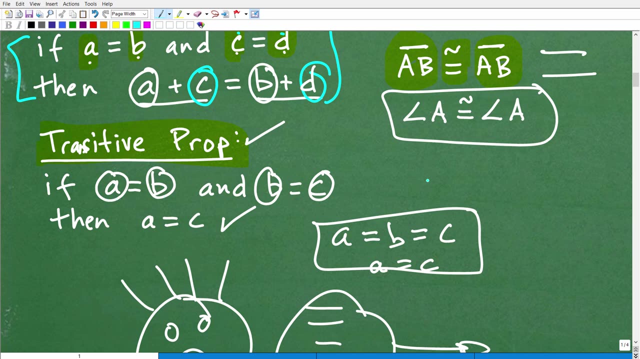 angle two: Why? Because of the transitive property. Okay, And to be more technically correct, you could put the transitive property of congruence Recall. let me go up here real quick. Remember what the transitive property is, And that is this: If a is equal to B, Okay, So here. 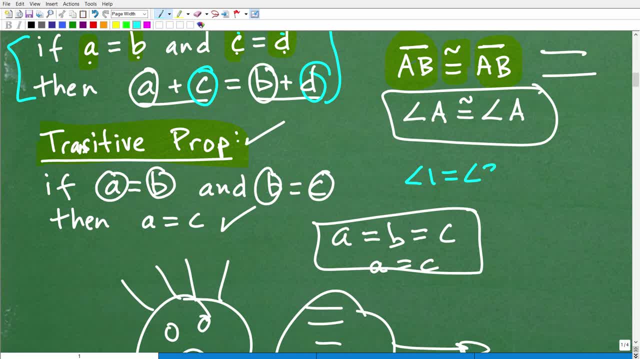 we had. if angle one is equal to angle three, which we already know, and angle three is congruent to angle two, Okay, Therefore, A is equal to C. So, in other words, angle one is congruent to angle two, And that's what we want. But that is a illustration of the 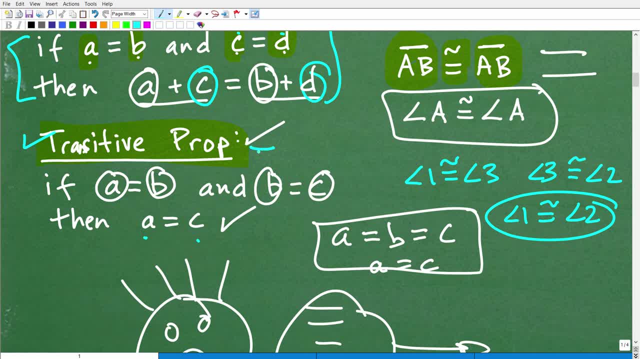 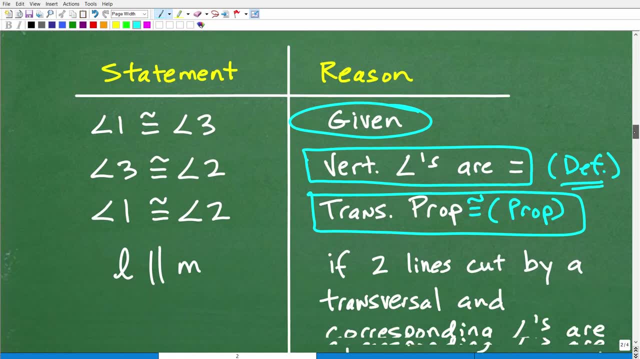 transitive property Now, because we're not using equal signs, we're using congruent signs. transitive property of congruence. Oh boy, Okay. So you know if you're struggling with proofs. you know there are, you know they're. they're like a little puzzle You got to figure out like. 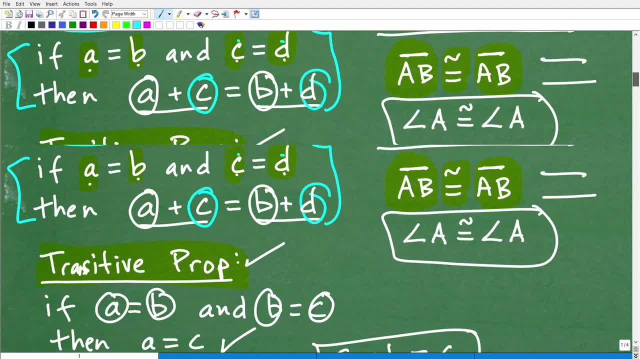 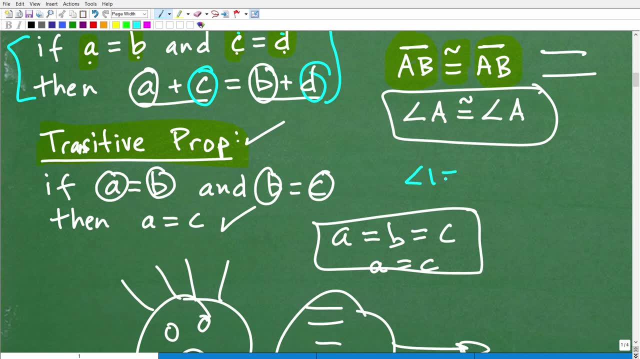 recall, let me go up here real quick- remember what the transitive property is, and that is this: if a is equal to b, okay. so here we had. if angle 1 is equal to angle 3, which we already know, and angle 3 is congruent to angle 2, okay. therefore, a is equal to c. so in. 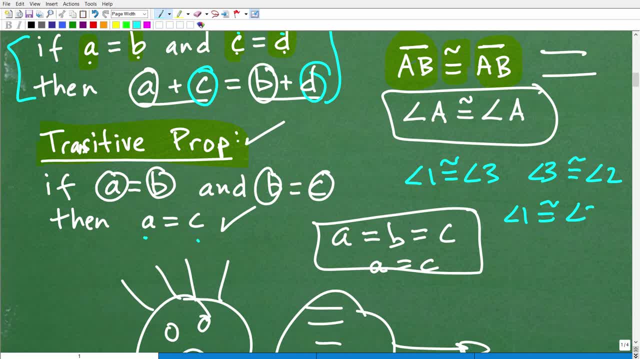 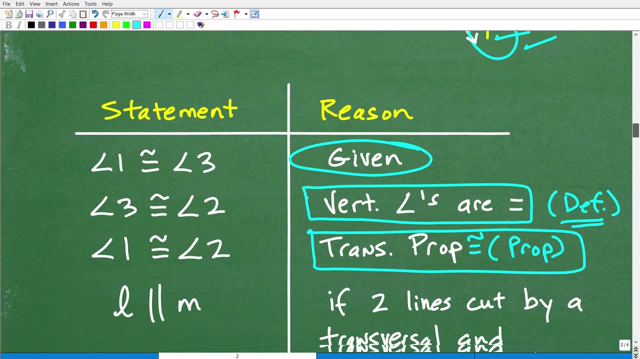 other words, angle 1 is congruent to angle 2, and that's what we want. but that is a illustration of the transitive property. now, because we're not using equal signs, we're using congruent signs. transitive property of congruence. oh boy, okay, so you know. if you're struggling with proofs, you know. 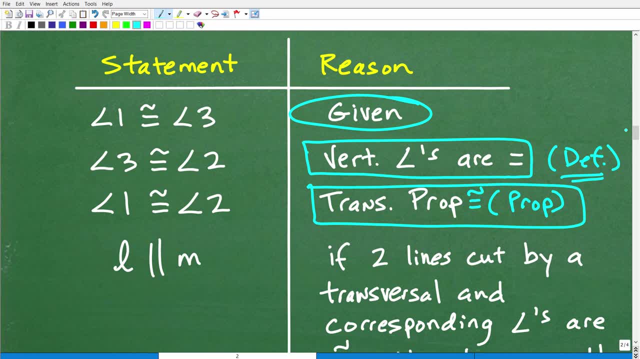 where to find out, where to find the right proofs. and you know there are. you know there are like a little puzzle you got to figure out, like a little rubik's cube cube or what cube rubik's cube gosh? i remember those things came out in the early 80s. they were driving people crazy. uh, typically people. 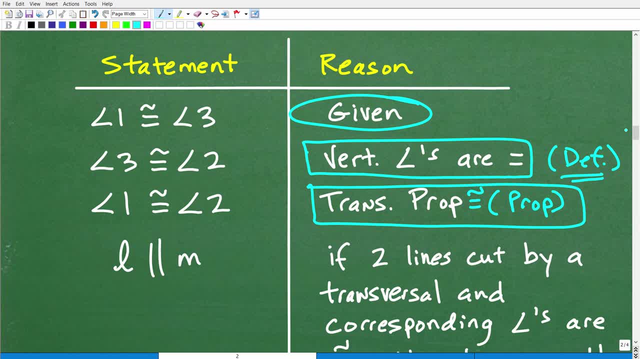 would just take them apart and put them together the right way. you can't necessarily do that with a problem like this, but you can get better at math and that's the whole idea here. okay, so transitive property. so we're pretty good to go. we've um, proved um or up to this point. angle one and angle two. they 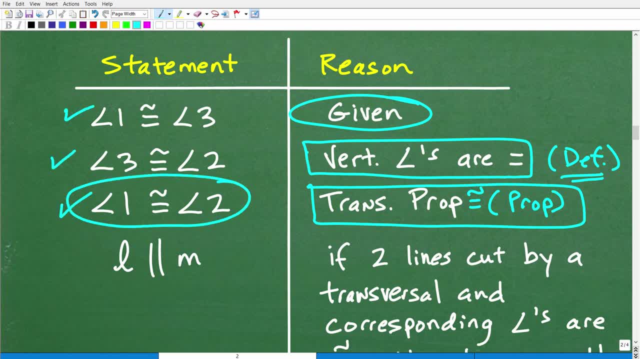 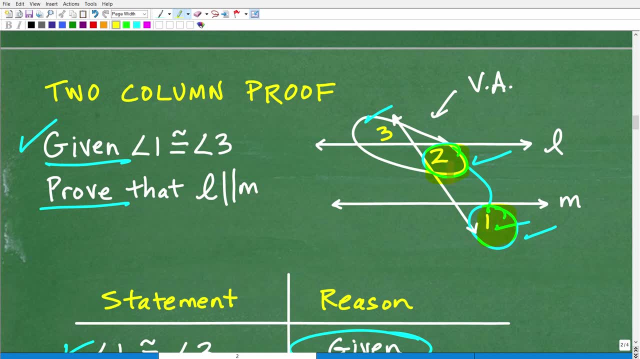 are, up to this point, angle one and angle two are congruent, and this is really kind of the secret to our kind of game plan here. as long as we could prove that these corresponding angles are congruent, well, that can only happen if the lines here, these lines formed with this transversal, are. 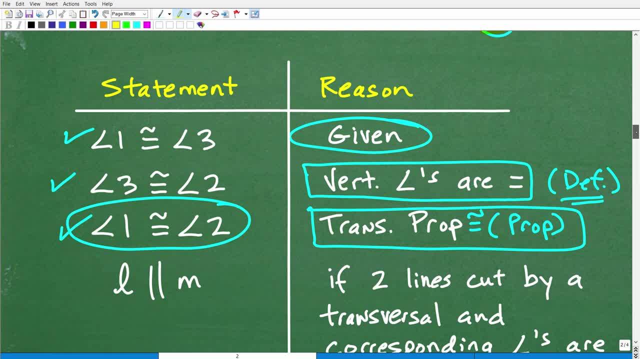 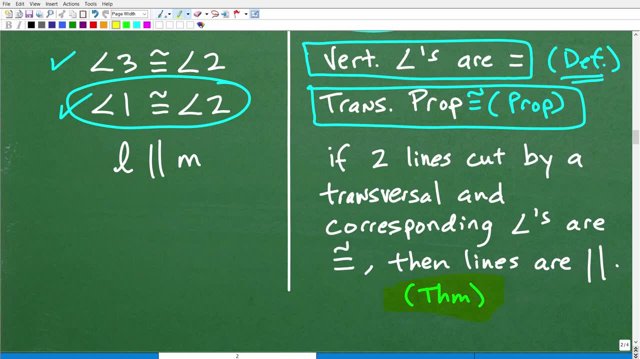 parallel, okay, but what says, what basically establishes that? well, we have a thing called a theorem that backs this up, and just to use a paraphrase, so now we can find, make our justification. hey, angle, uh, i'm sorry, line l is parallel to line m. if i've been saying angle, i apologize. i am. 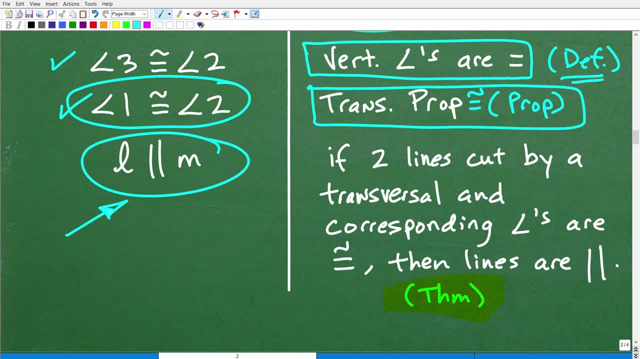 speaking a lot, a lot. i'm trying to stay focused here. so even myself doing you know, teaching this is, you know, can be challenging sometimes. so line l is parallel to line m. okay, that's my final conclusion, but i got it back to you. it says: if two lines cut by a transversal, okay, and the corresponding angles are congruent. 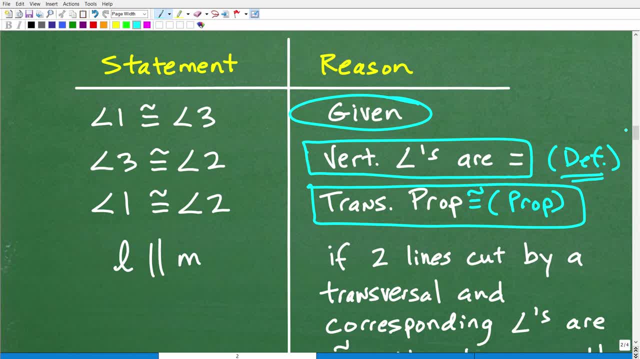 little Rubik's cube, or what cube Rubik's cube Gosh? I remember those things came out in the early eighties. They were driving people crazy. Typically, people would just take them apart and put them together at the right way. You can't necessarily do that with a problem like this, but you can get. 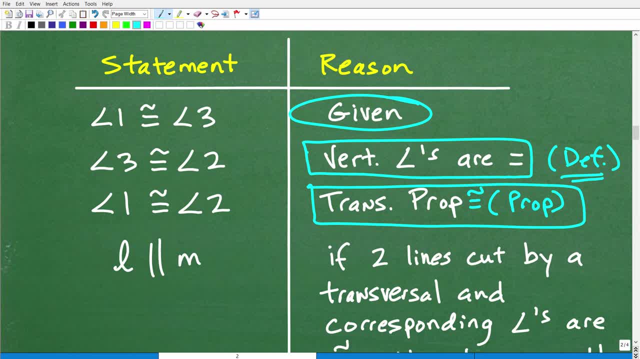 better at math And that's the whole idea here. Okay, So transitive property. So we're pretty good to go. We've proved um are up to this point. angle one and angle two are congruent, And this is really kind of. 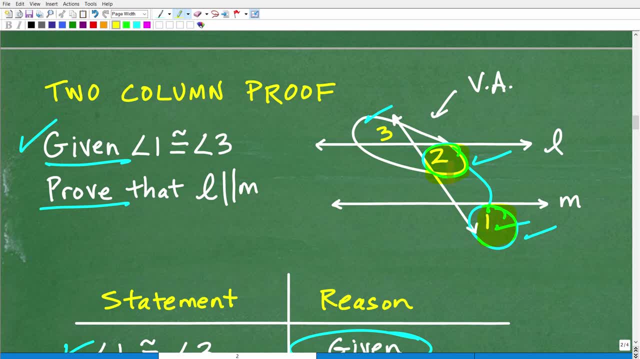 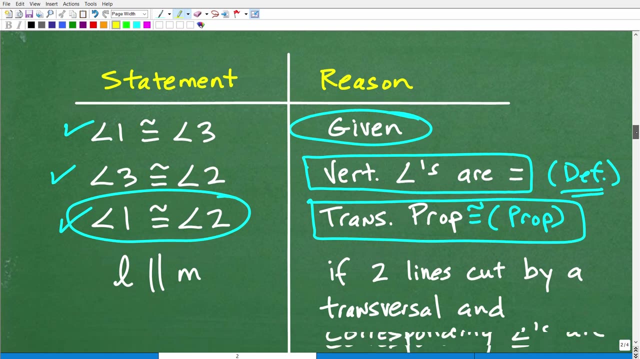 secret, uh, uh, to our kind of game plan here, As long as we could prove that these corresponding angles are congruent. Well, that can only happen if the lines here, these lines formed with this transversal, are parallel. Okay, But what says, uh, what basically establishes that? Well, we have. 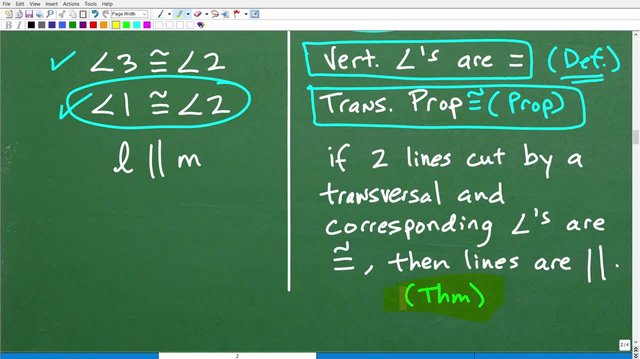 a thing called a theorem that backs this up, and just to use a paraphrase. So now we can find, make our justification: Hey, angle, uh, I'm sorry, Line L is parallel to line M. If I've been saying angle, I apologize. I am speaking a lot, A lot of. I'm trying to. 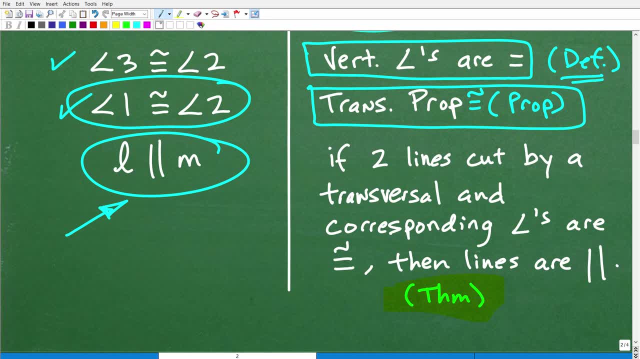 stay focused here. So even myself, doing you know, teaching us is, you know, it can be challenging sometimes. So line L is parallel to line M. Okay, That's my final conclusion, but I got to back it up with a theorem. It says: if two lines cut by a transversal, okay, And the corresponding angles. 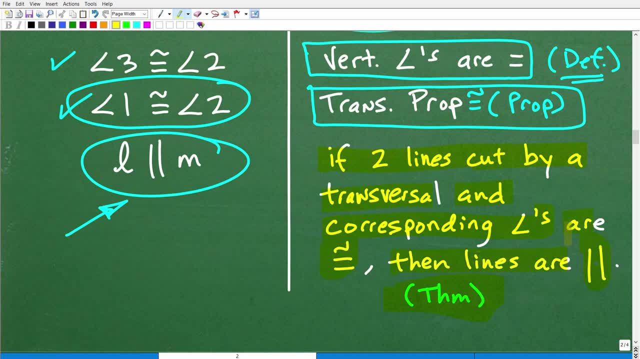 are congruent, then those angles are congruent. So line L is parallel to line M. Okay, So line L is parallel to line M, If you can, and it's a good proof that those lines are parallel. Okay, That those lines are parallel. And? um, this is an example of constructing a geometric proof. Okay, 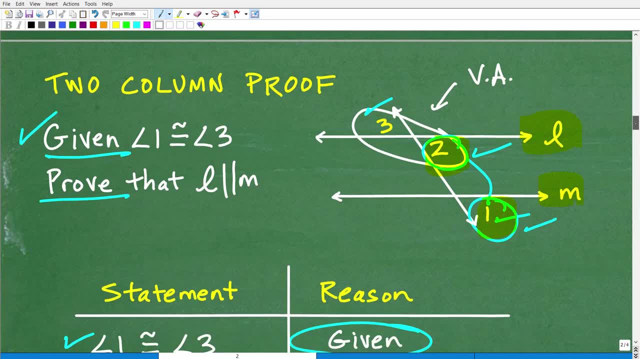 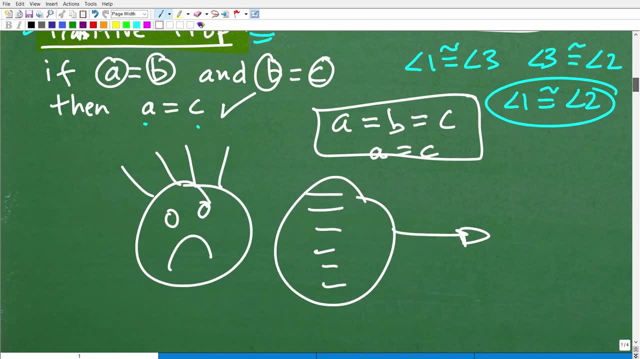 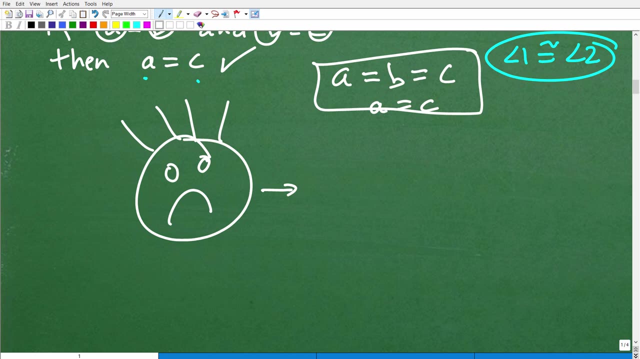 It's pretty involved, All right, No doubt about it, And if you're having, you know, uh, problems doing proofs, that's pretty normal, Okay, Even for very good students. but hopefully this little video here helped you kind of go from this little face to let's kind of give it a little bit of a 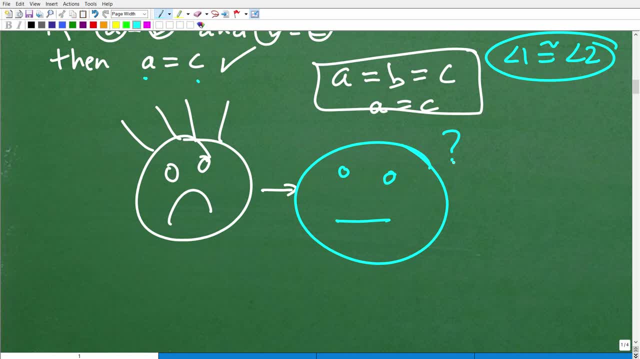 nice little picture, Okay. So this is a little video that I'm going to show you And I'm going to face here, maybe to like this face. be like: okay, i think i can do this. i can assure you, if you continue to practice, you'll end up with a nice little happy face. you'll be like: i am so smart.